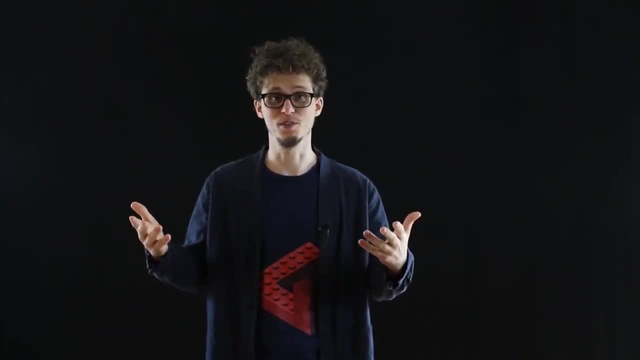 turns out, human beings actually have many more than just those five, And something like touch turns out to be a very complex package of many different senses bundled together. We have the ability to feel pain, We have the ability to feel temperature, We have a sense of balance, We have 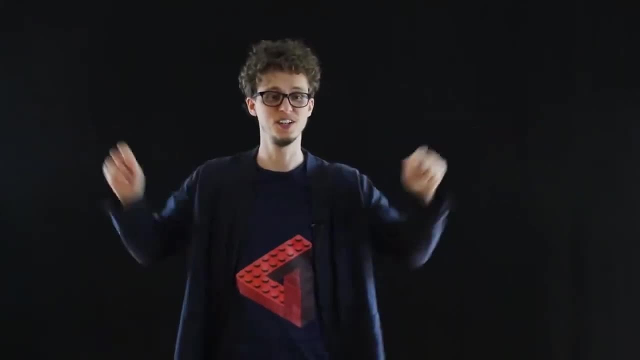 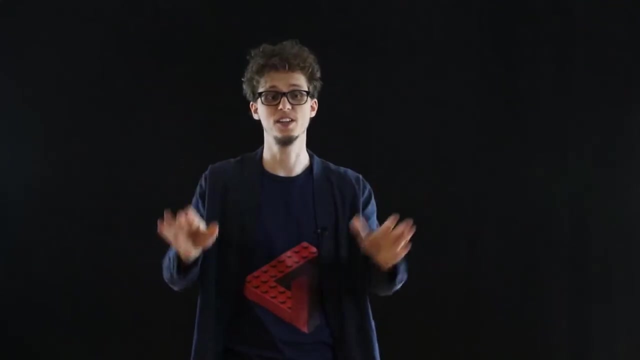 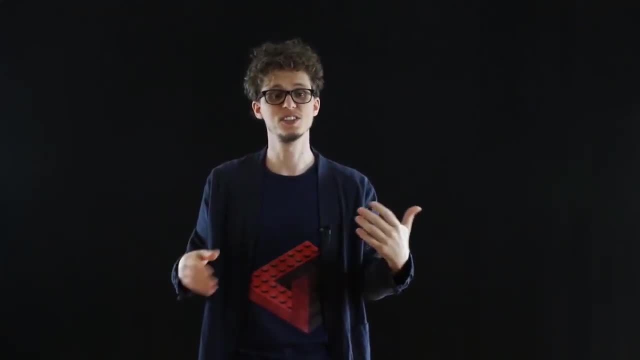 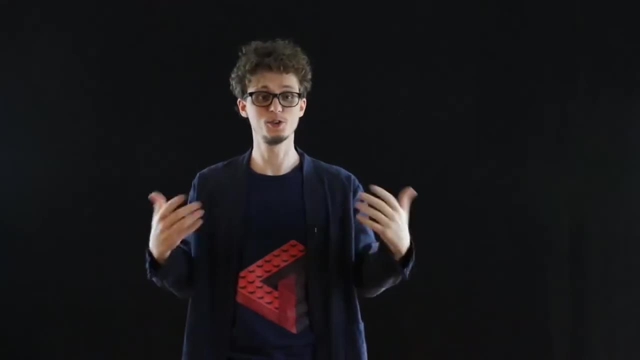 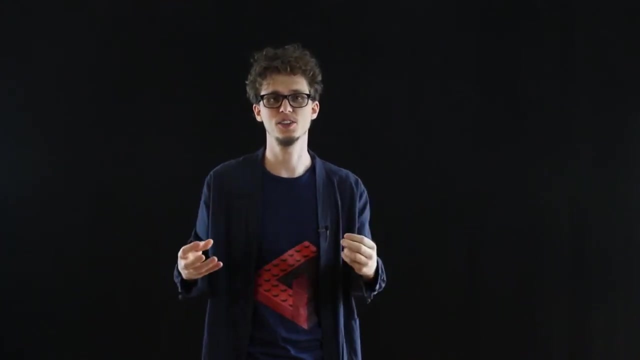 them. That's its own kind of sense. We have senses like feeling hungry or feeling full, The sense of having a full bladder or needing to use the bathroom. Those are all senses. All of those represent certain kind of information that enters into our brains via those outside channels that 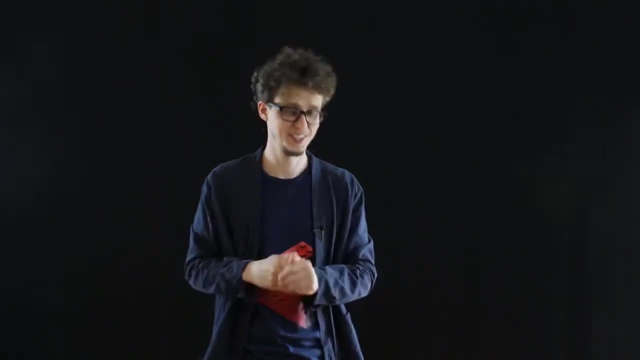 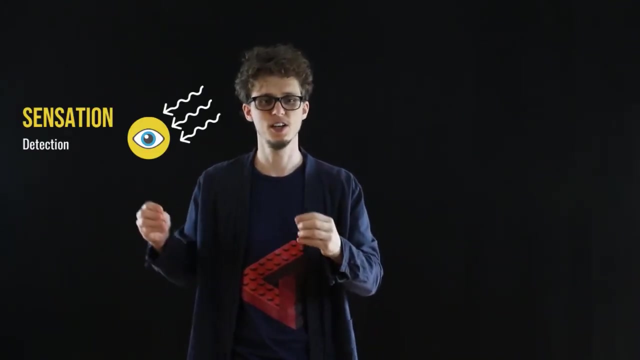 tell us something about the world or something about our own body, And we have a sense of our own body. And each type of information coming from each of our senses goes through these two stages of sensation: that raw detection, getting the information into our brains, and then 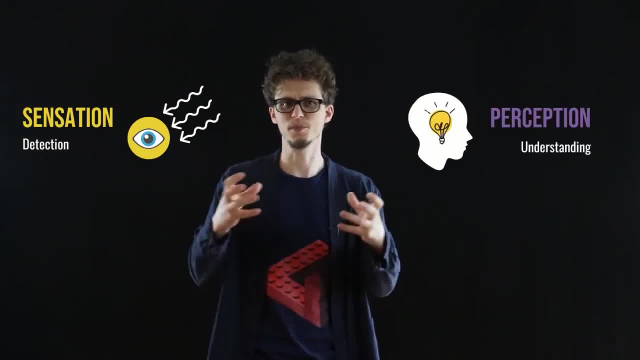 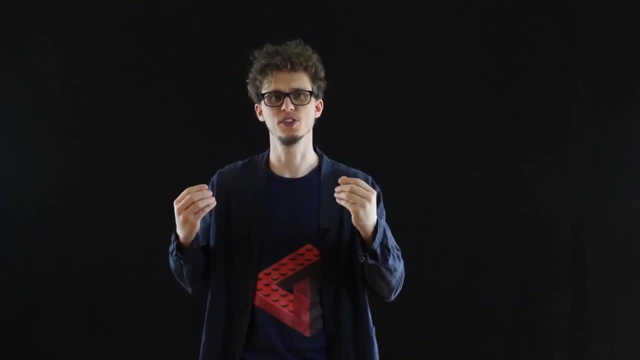 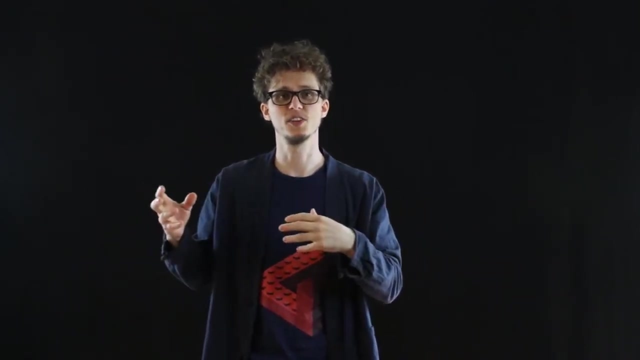 perception, using the information, interpreting it, building something out of it, making sense of it. The first step in sensation after we get that information through our sense organs is the conversion of that information from its raw form to some form that our minds can comprehend. And 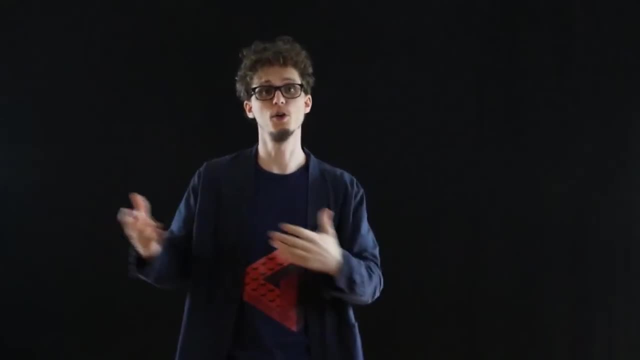 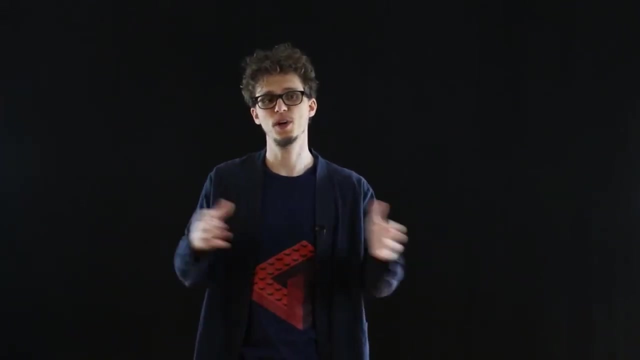 we talked about this when we talked about mental representation, that in order to know things about the world, we have to take information from the outside world and convert it into a format that's readable by our minds. This process is called transduction. You can think about it sort. 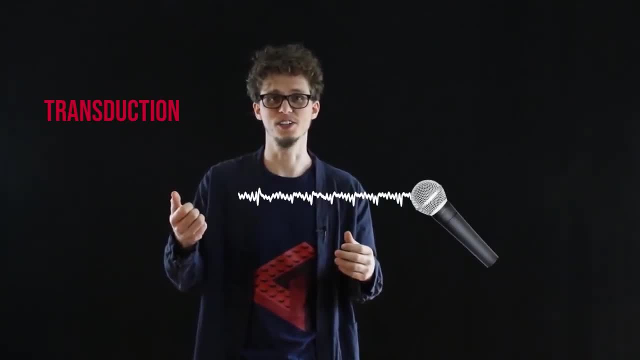 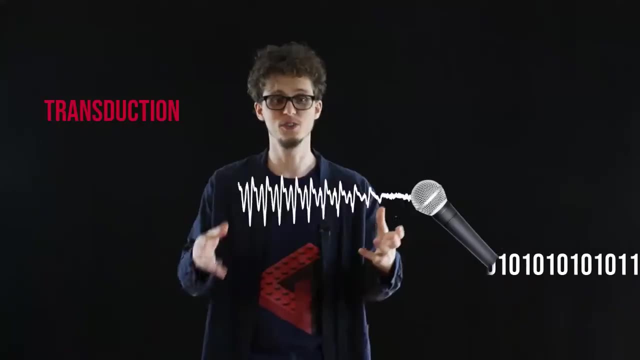 of the way a microphone works. A microphone takes a sound signal, compressions of airwaves, and it turns it into an electrical signal, an electrical signal that you can then run through an amplifier or into a computer to record it. Same thing's happening in our minds. 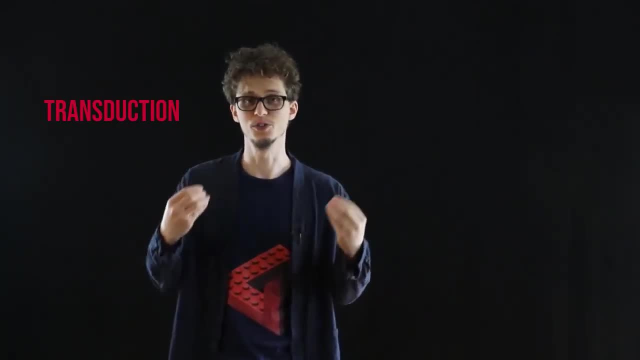 Our sensory organs, our eyes and ears, our nose, our taste buds. they're all recording certain kinds of information, But the way in which they record it has to be translated into a form that our brains can make use of, So that transduction process takes things from the outside world. 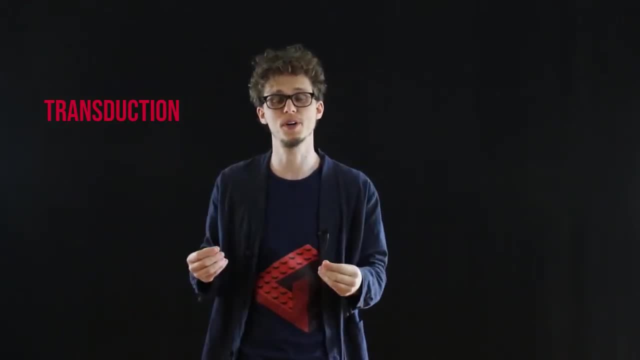 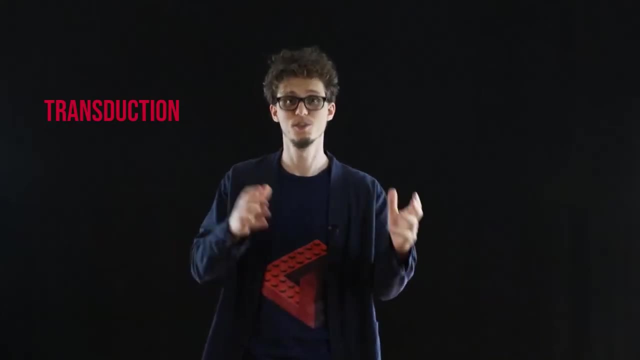 through our senses and converts it into a form that's readable to a human mind, And that always has to be step number one. Before we can get to perception, before we can understand what's going on in the outside world, first we have to take that information and transduce it into a form that's 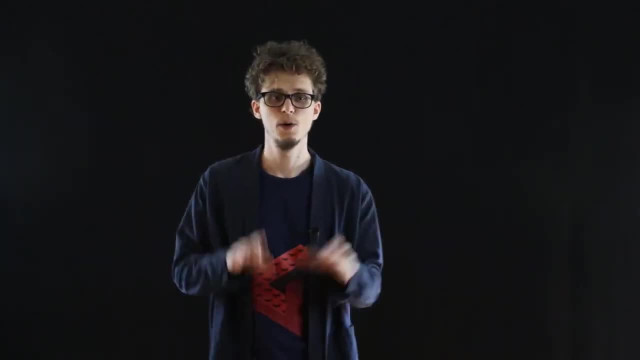 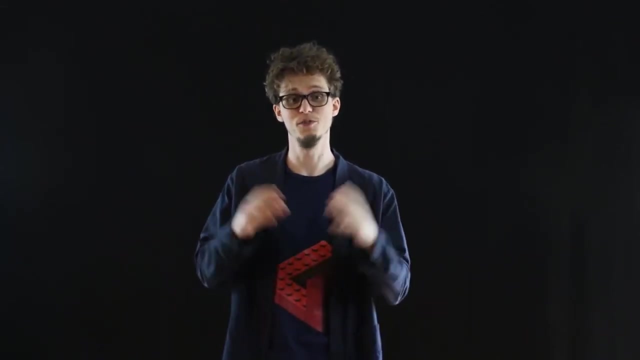 usable to our minds. I want to focus now on one sense in particular. I want to focus on vision, because this has been a really rich resource area for cognitive science. Vision is the most well understood of our senses And in a lot of ways it's sort of our primary sense, It seems to be. 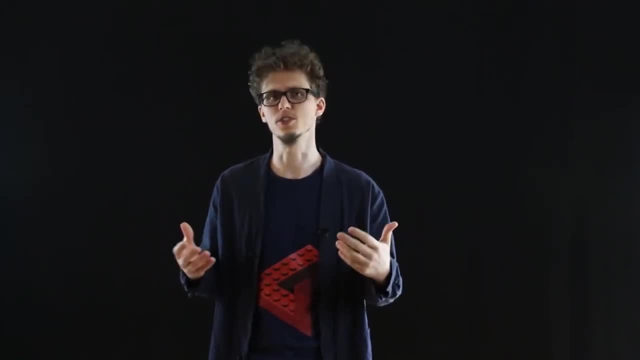 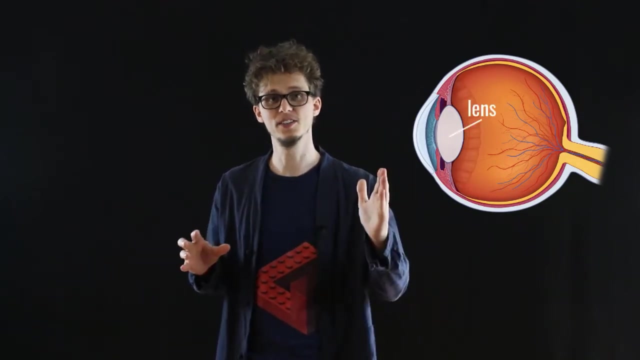 the one humans rely on the most for navigating the world and making decisions, And vision starts at the eyes. So let's talk about the anatomy of the eye. The eye is basically a big orb full of liquid. On the front end of it is the lens through which light passes. We have an iris. 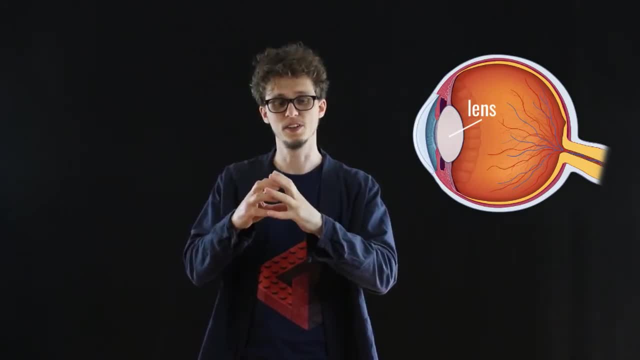 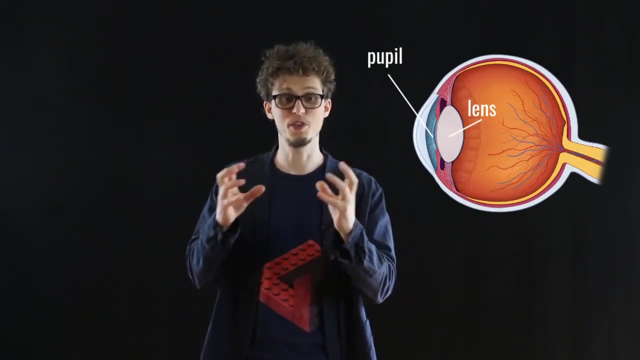 which is a muscle that can contract or expand, And the opening in the middle of the iris is the pupil. We see a pupil as a dark spot in the middle of our eyes. We think of it as kind of a thing itself, but it really isn't. It's just a hole, It's the aperture. If we think of an eye as being sort of 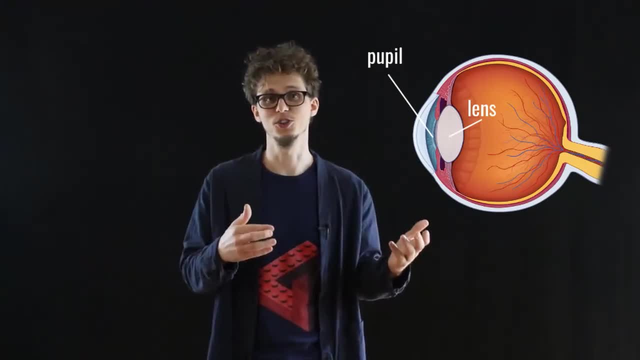 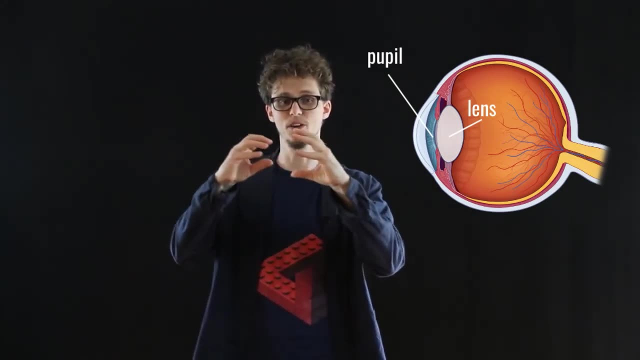 like a camera. The camera has a lens. The camera has a shutter. A camera has an aperture, Same with the human eye. We have the lens, We have the aperture, The camera has a lens. The camera has a lens. We have an aperture, which is the iris, which can become big or small to let in varying. 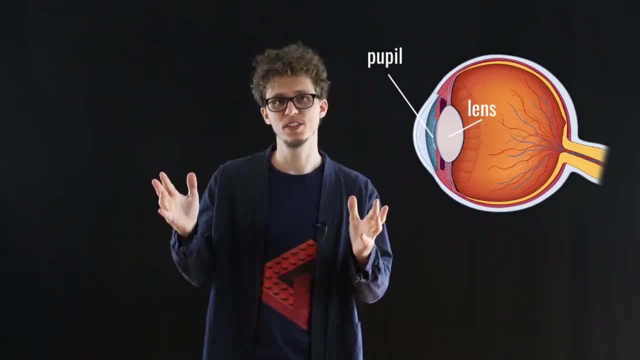 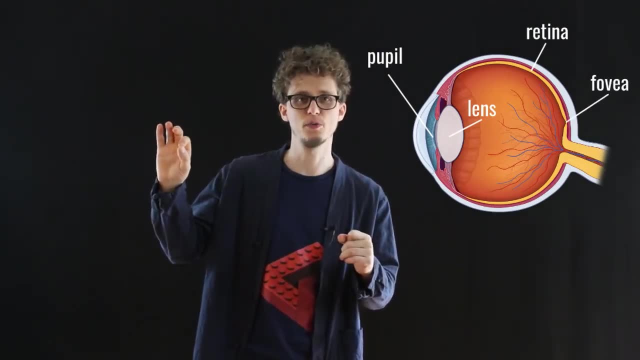 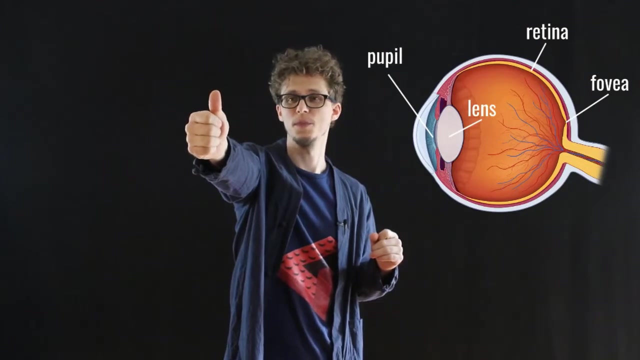 amounts of light And it's a layer of photoreceptive cells that react to light. that line the retina And we have a tiny focal area called the fovea at the back of the retina. That's the area of highest acuity. If you put your hand out in front of you like this and you look at your thumbnail, that's 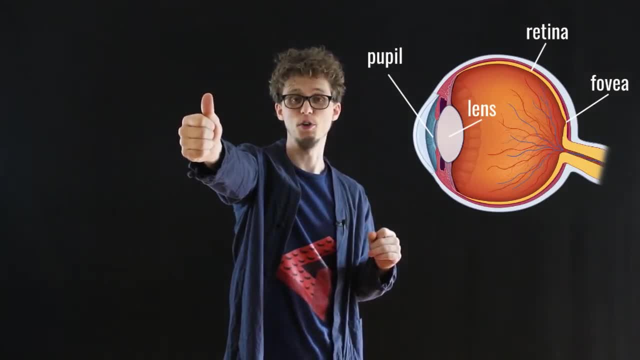 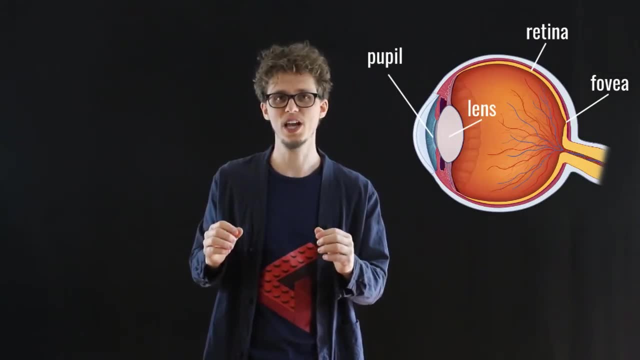 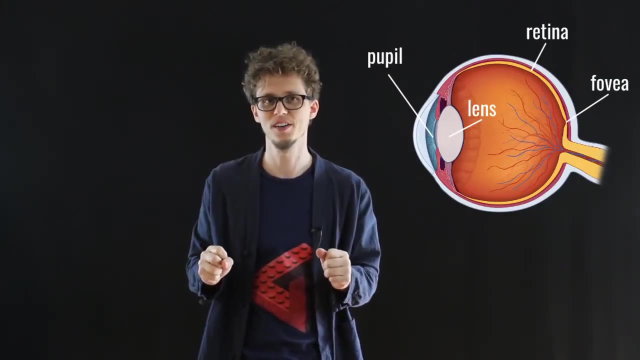 about the size of the field of vision that the fovea covers. So the area of our field of vision that has the highest acuity is a very, very small area. We only have very detailed, in-depth visual information for a very tiny area of our entire visual field at any one time. Somehow we take that. 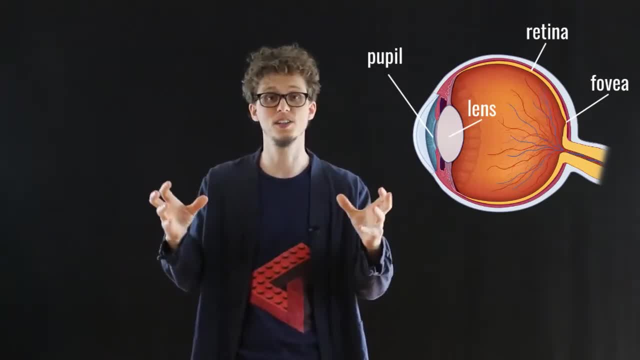 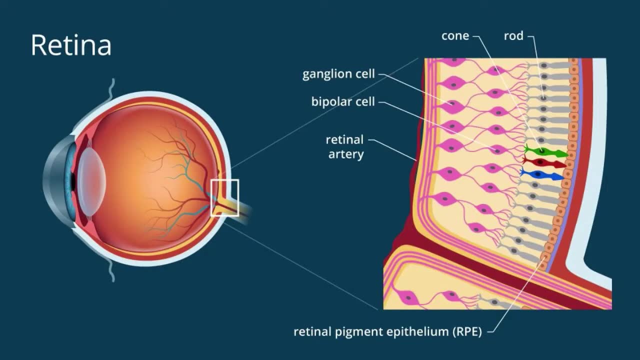 tiny information and we scan our environment continuously and stitch it into a highly detailed image of the outside world. There are two main types of photoreceptive cells on our retina: Rods- which, true to their name, are shaped like rods. These work better in the dark. They don't. 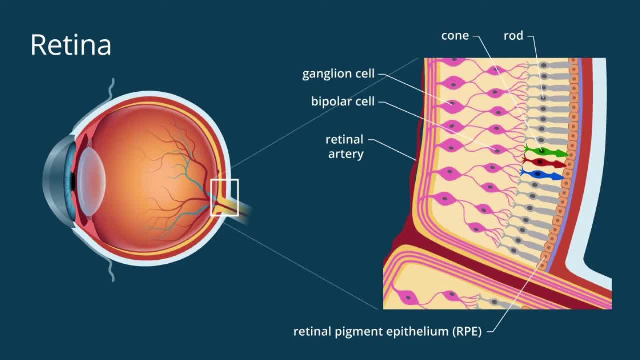 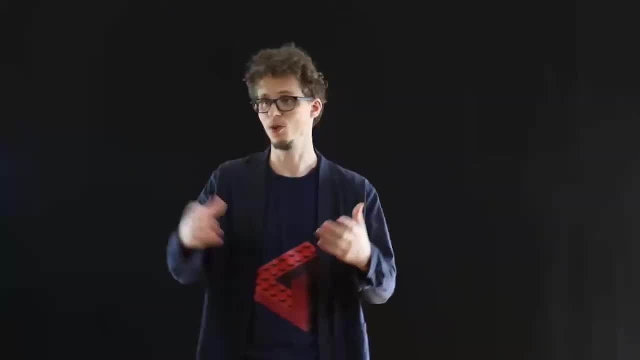 require quite as much light. They don't require as much light. They don't require as much light In order to work, But they can't distinguish colors and they have much lower acuity. So you may notice at night. you have a hard time discriminating different colors If you walk in a parking lot. 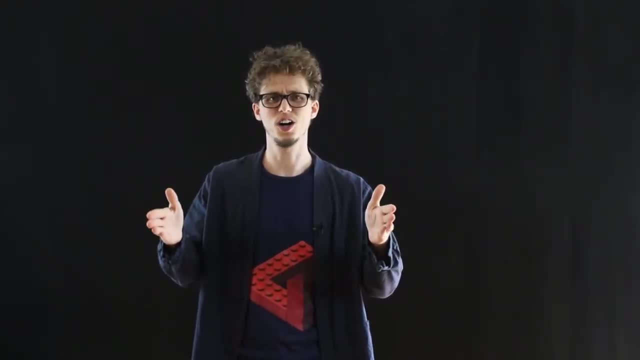 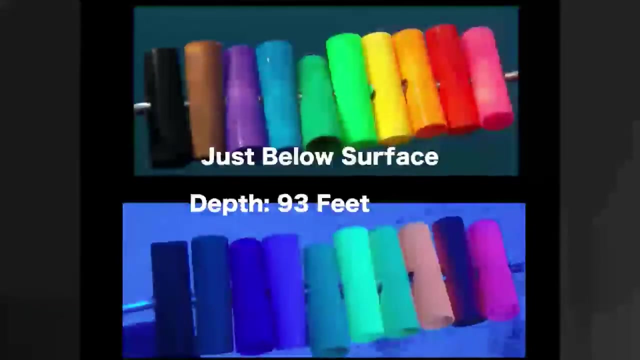 after the sun is set it's hard to tell which cars are which color. They all kind of just look dark. Is it blue or red? I can't quite tell. Same thing happens if you dive under the water in the ocean. The further down you go, the less light will reach you and the more various colors will start to just. 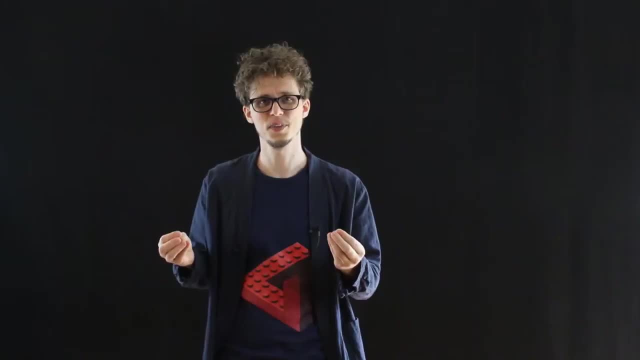 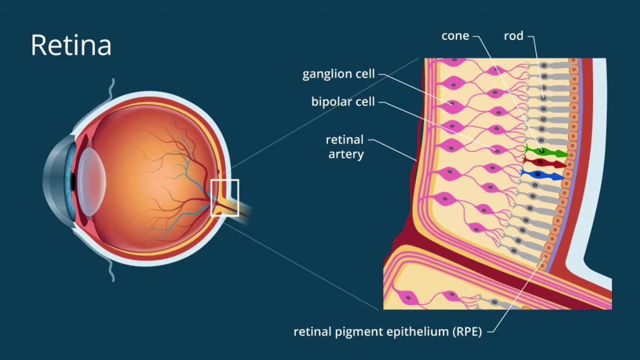 look dark, That's because we're relying on our rods, and our rods just do not have the capacity to distinguish one color from another. The other type of photoreceptive cell we have are called cones. They are shaped like cones and they work much better in light. They require a lot more light. 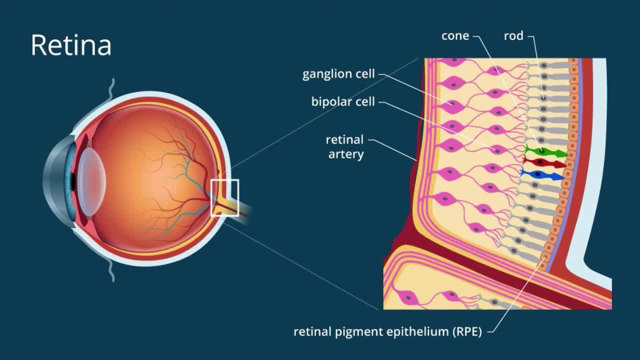 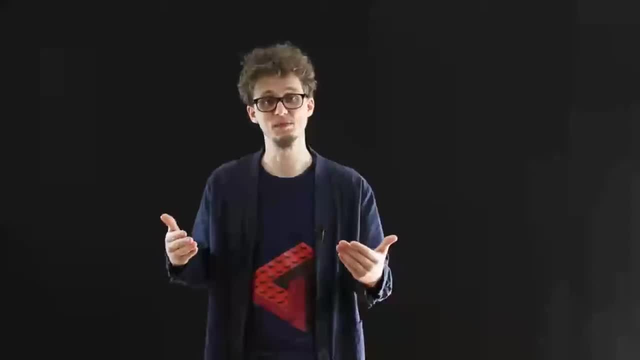 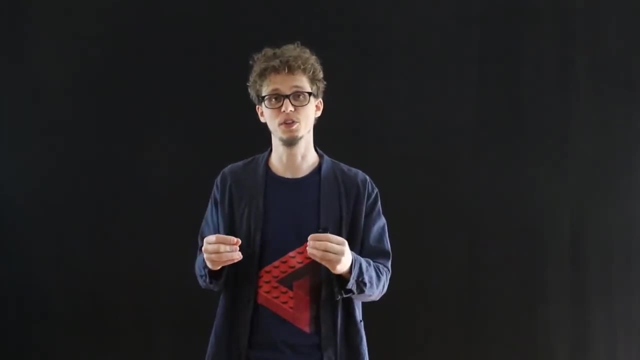 in order to detect an image, but they can distinguish color and they have much higher acuity. So cones are the cells that we rely on in daylight, And it's the cones that are at their densest in our phobia, which gives us that high visual acuity. 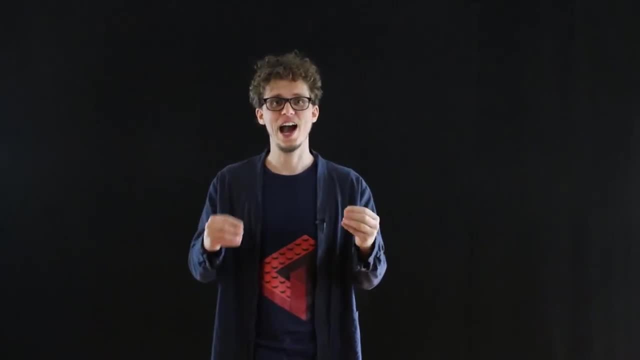 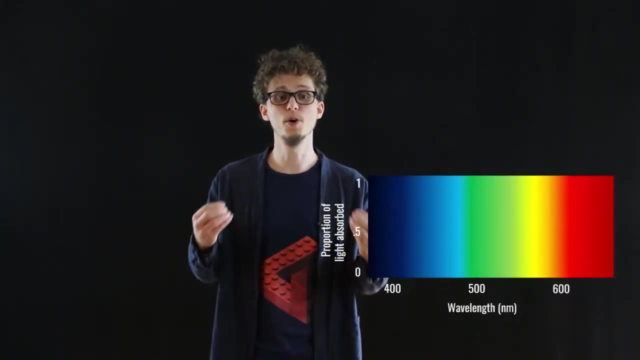 Each type of cone has an activation function that determines how activated or how excited it gets by any particular wavelength of light. So the short cones are most excited by wavelengths in the lower end of our visual spectrum, around 400 nanometers. The medium cones are much more excited by 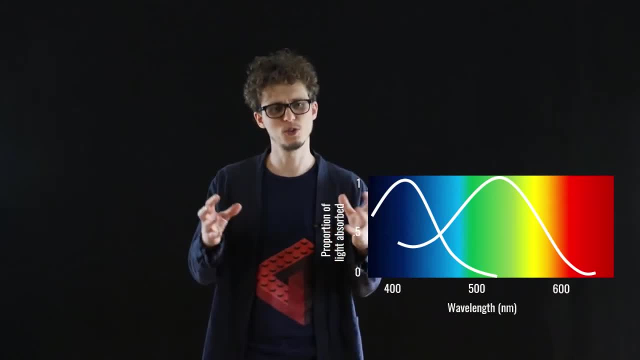 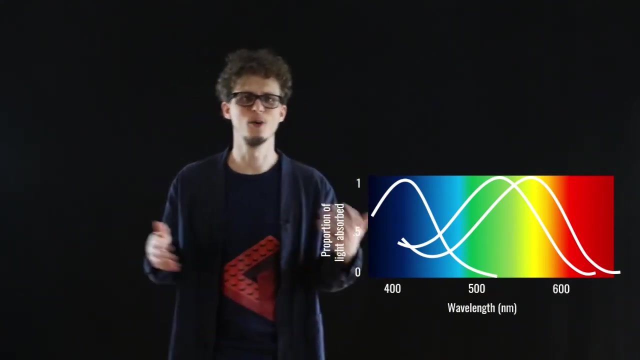 wavelengths of light around 550 nanometers In sort of the green-yellow area, And the long cones are mostly excited by wavelengths of light closer to 600 nanometers, firmly in yellow territory. So how do we see things like red or orange or all of these other colors? Well, it's actually. 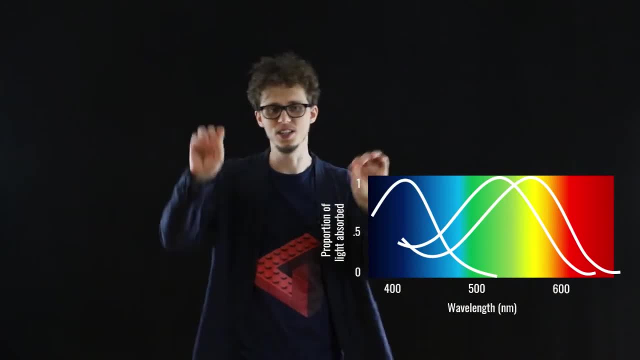 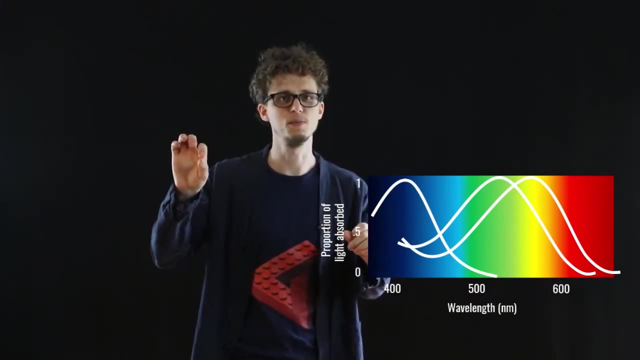 the combination of all three of those cells responding in different degrees. that gives us our sense of color. Pure red will activate the long cones much more than the medium and not at all. actually, A color like yellow is going to activate the long cones and also the medium cones, but 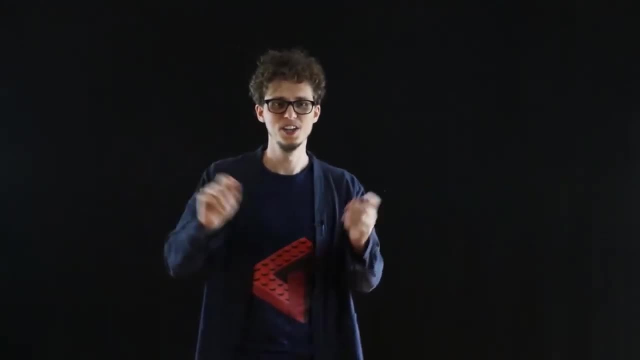 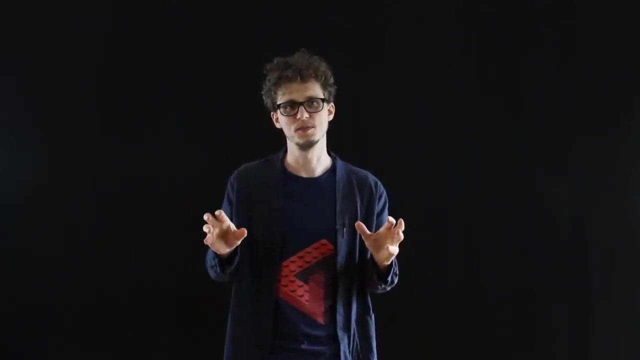 it will activate the long ones a little bit more than the medium ones. So just charting all of these different values, how excited each cell gets, we can derive every color that we can experience, And in fact this can give us an experience of colors that in 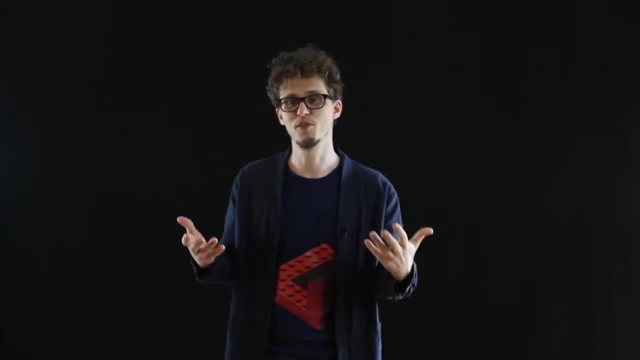 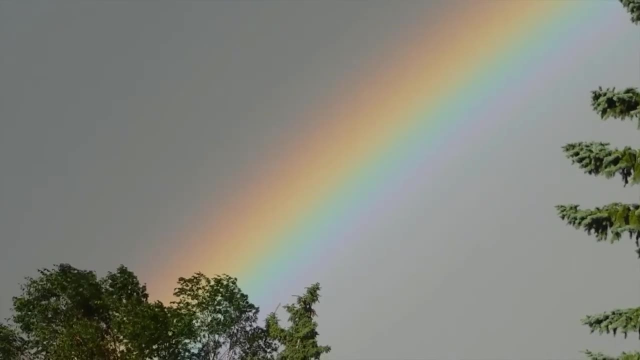 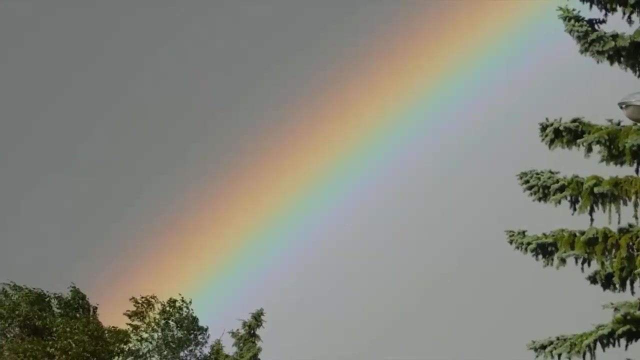 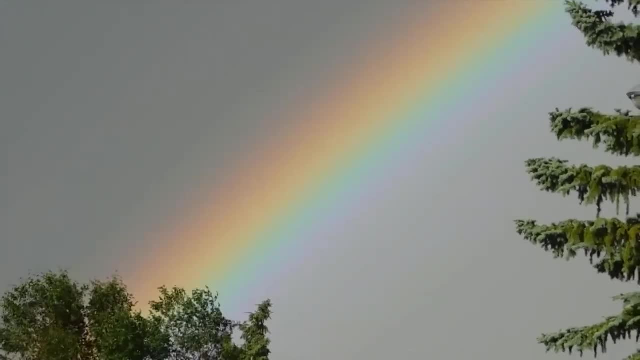 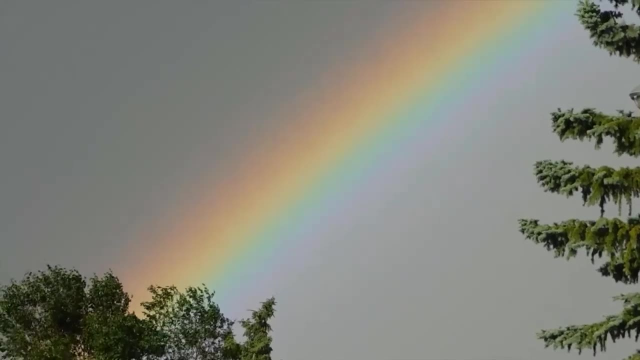 coloration, of the coloration, of the coloration. Now, when I look at a rainbow, you might notice- well, wait a minute. I can see where red turns into orange, Orange turns into yellow, yellow turns into green, green into blue, blue, into. 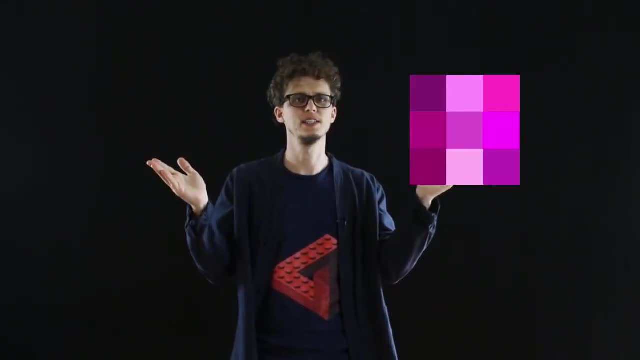 maybe a indigo or purple, but I don't see any region where purple blends back into red. A rainbow only goes one way, It doesn't loop back on itself. So where in the visual spectrum of light are those purplish, blueish colors? And the truth is: 감사합니다. Nowhere. they don't actually exist, not in a physical sense. Our ability to perceive a bluish-purple color is an artifact of us perceiving blue and purple at the same time. It's an illusory color. 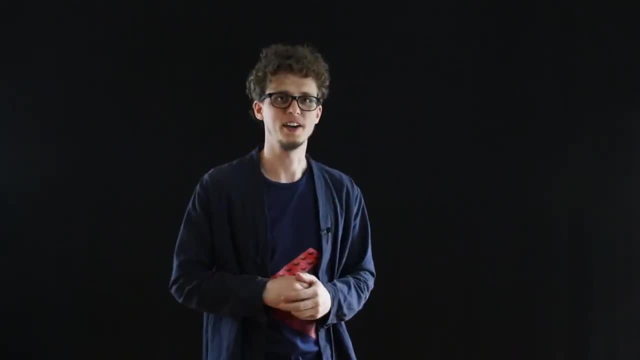 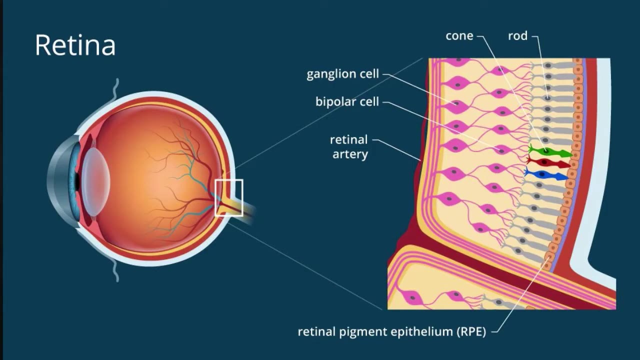 Maybe that's why I like them so much. Here's one more wacky fact about the retina. We know the retina is lined with those photosensitive cells that detect light and give us our experience of the things that we're seeing. but there's something a little bit weird about it. 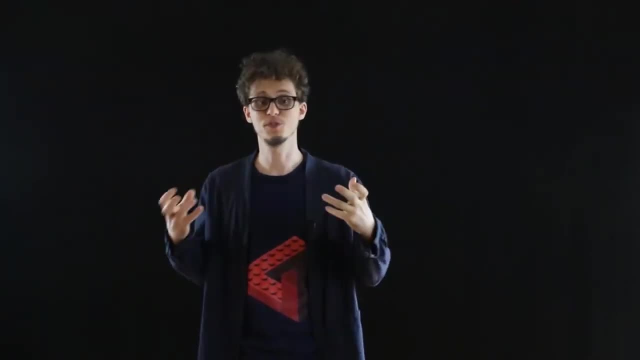 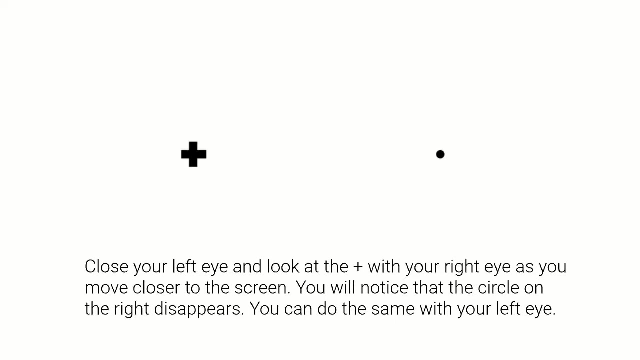 You may have heard that we have a blind spot and you can test this for yourself. You may have seen something like this: You look at a cross on a screen and there's maybe a dot, and if you're looking at the right distance, the dot will disappear. 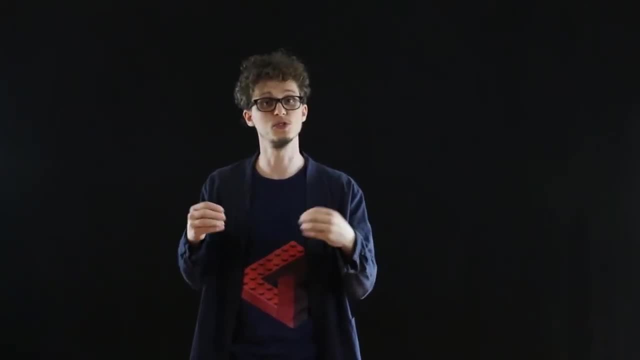 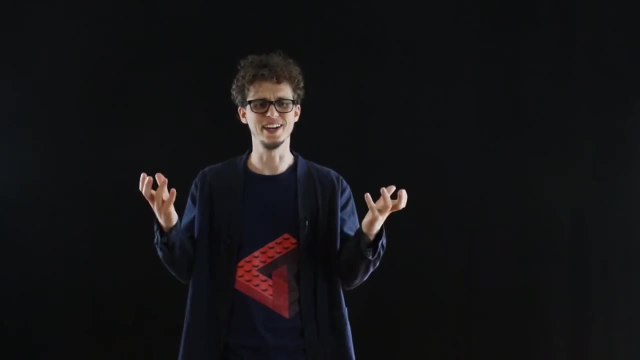 That's because there's a part of our retina that actually doesn't have any rods or cones at all. It's a blind spot. There are no photosensitive cells in that area. Why? Why should we have a blind spot? It seems like a huge limitation. 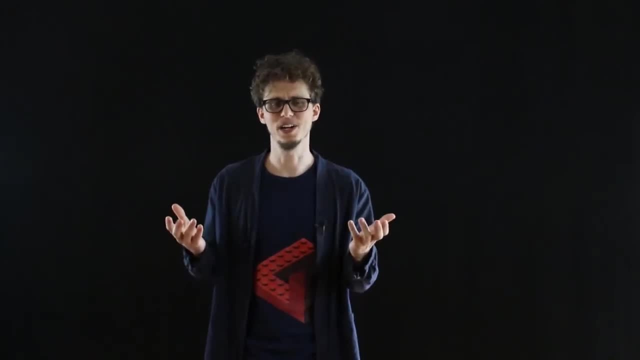 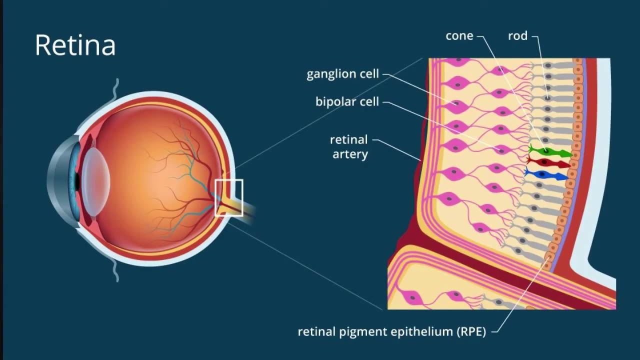 Now, I don't know, Or a big design flaw- Who would design an eye with a blind spot? It turns out there's a good reason that we have a blind spot. The blind spot is the area of the retina where the optic nerve connects to all of those photosensitive. 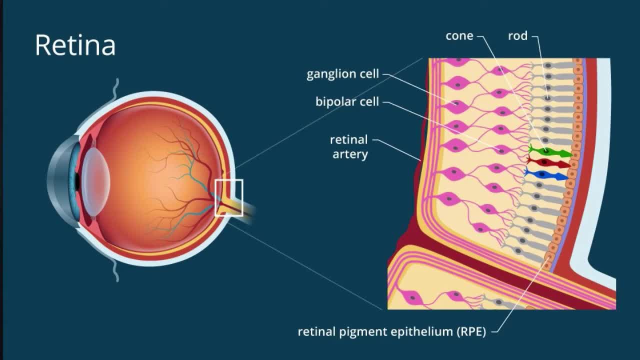 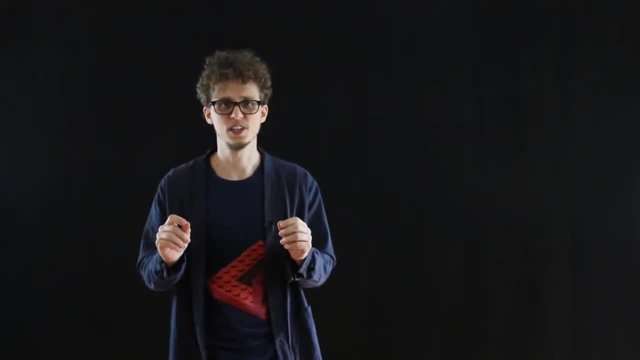 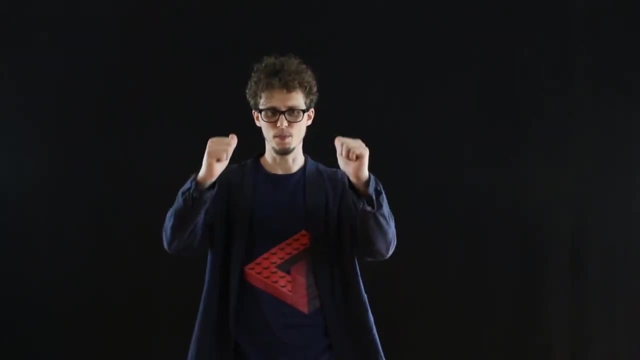 cells. But why should it need to puncture through the retina to do that? This is where the story gets really wacky. All of those photosensitive cells that line our retina. they're actually backwards. The part that detects light points inside, towards the back of our skulls. 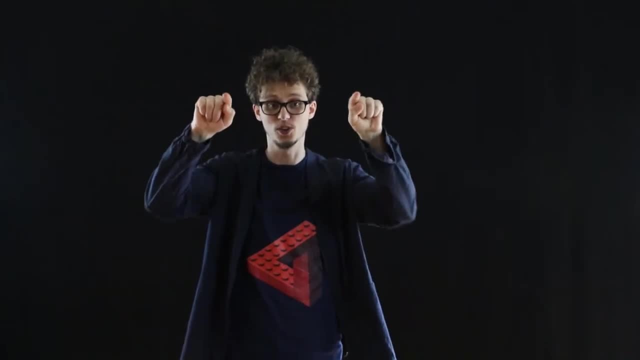 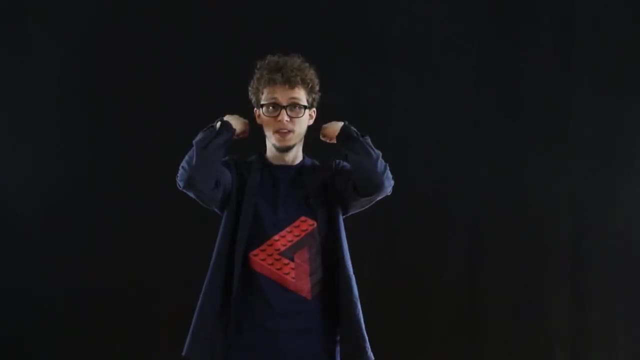 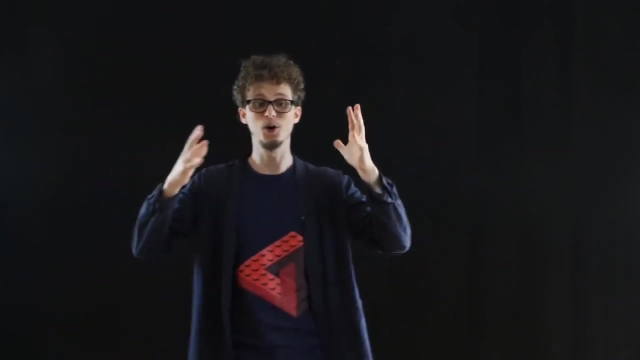 And the part that sends the electrical signal to our brain points forward towards the front of our eyes. So all of those cells have to double back and then pass through the retina to pass that information through the optic nerve into the brain. I don't know who came up with this, but it's totally bizarre. 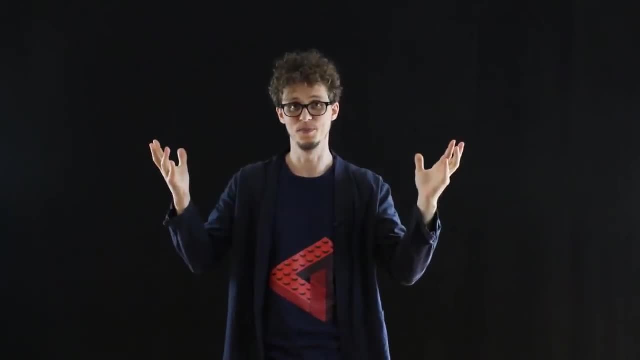 It's bonkers: The eye is built backwards And it just so happens that not all works out the same way. I don't know who came up with this, but it's totally bizarre. It's bonkers And it just so happens that not all works out the same way. 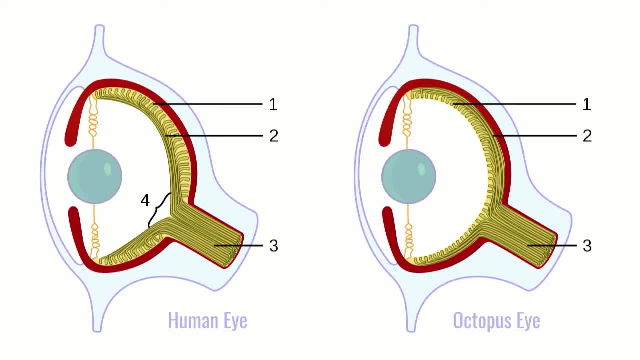 And it just so happens that not all works out the same way. Organisms have this structure: Cuttlefish, octopus, squids, cephalopods. they have very well developed eyes too. They also evolved separately from us, and their eyes, in my opinion, are much better designed. 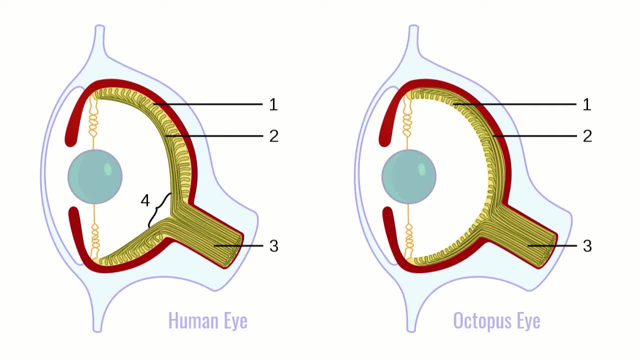 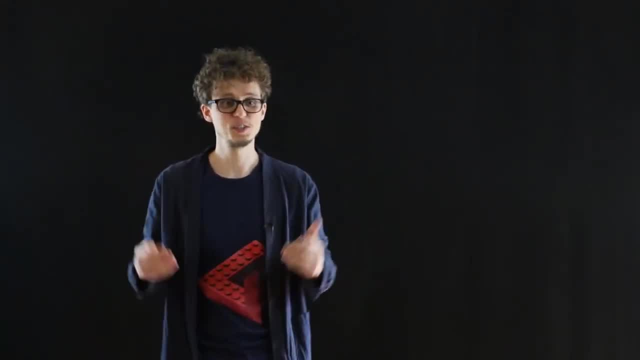 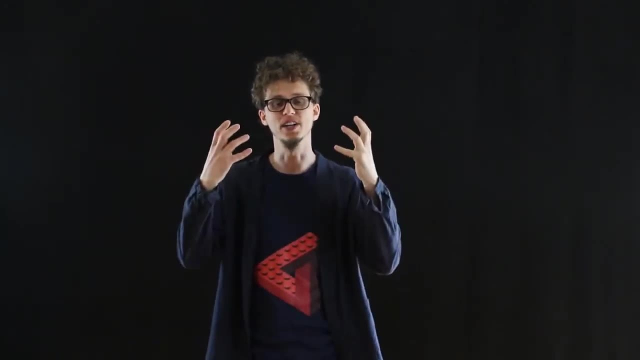 They don't have a blind spot Because their retinas are designed the right way around. This always cracks me up- Just part of the fun of being a human being. you've got backward retinas. Okay, What happens to that visual information once it hits the retina? 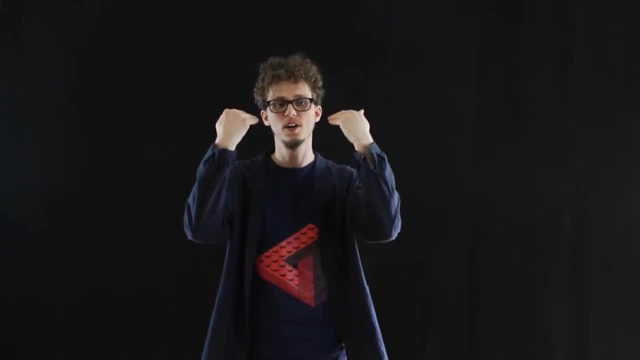 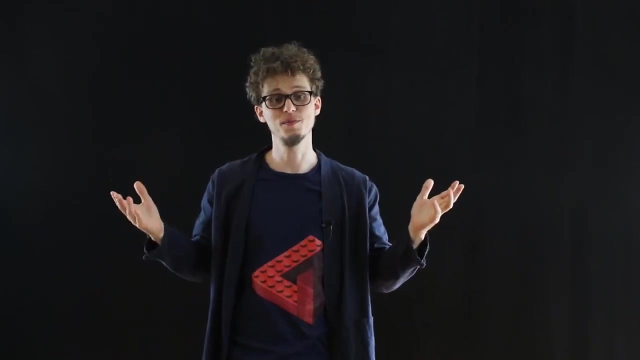 It's transduced into an electrical signal and then it flows on the optic nerve out of the eye. Where does it go? The optic nerve follows a pathway through the lateral geniculate nucleus to the visual cortex In another one of those wacky bonkers kind of things, the visual cortex where we process. 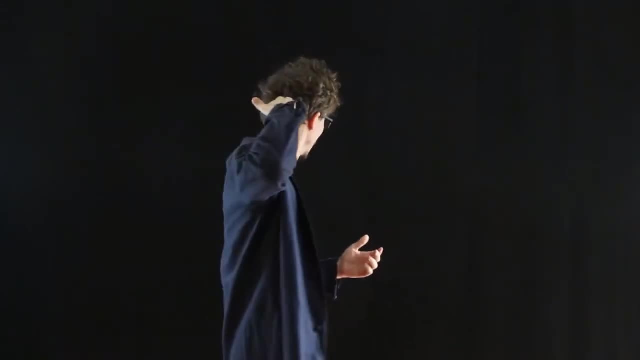 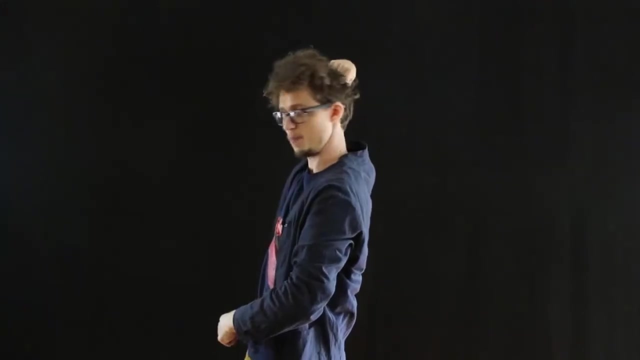 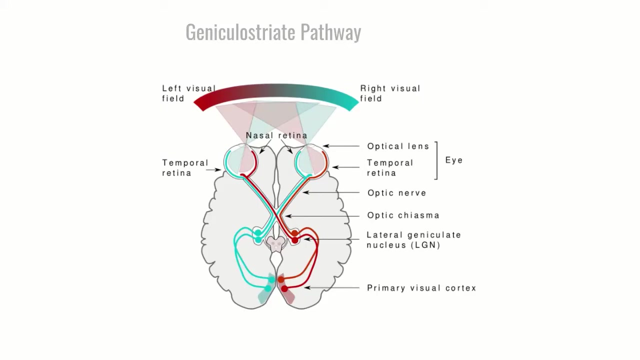 all of our visual data is in the very back of our brains, So the information flows from the eyes across the hemispheres to the back of the brain in V1.. This is called the geniculostriate pathway and it's the primary pathway that our brain 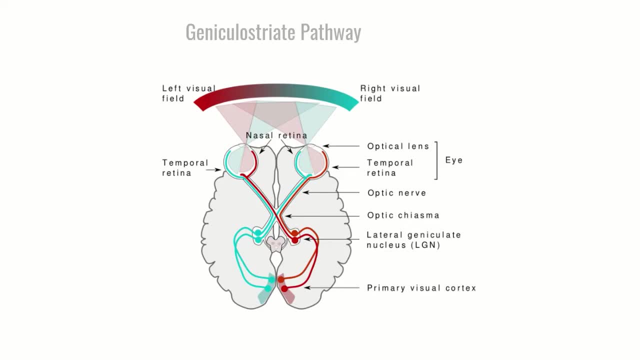 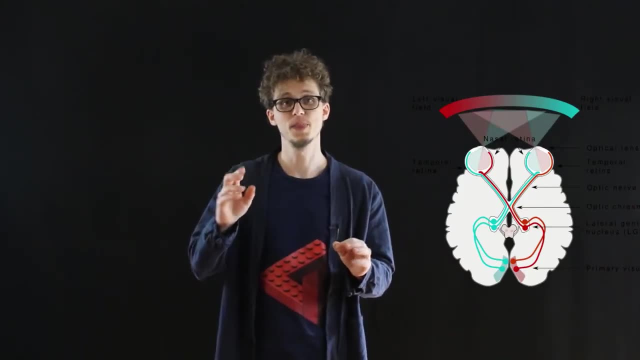 uses to process visual information. And there's one more wacky fact about the way this is wired, and that is that we can separate our field of vision for each eye into two halves: A right visual field and a left visual field. So, even closing one eye, you'll still have a left half of your visual field and a right. 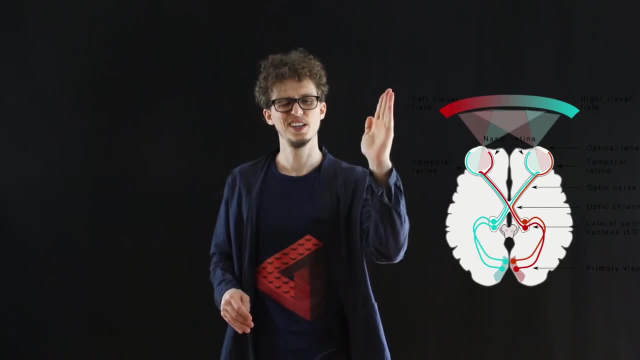 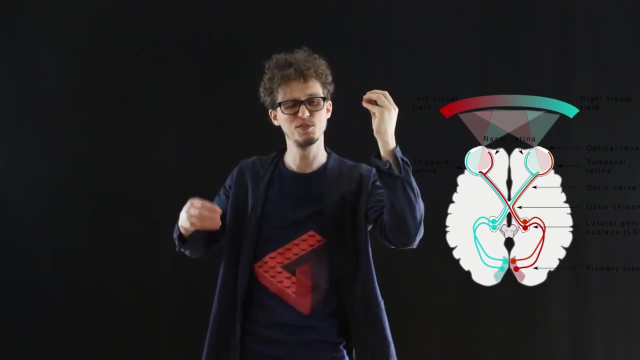 half of your visual field And the left half of your visual field, all of that information that goes into your eye and triggers your retina and goes into the optic nerve, is going to be processed in the right hemisphere. So your left visual field for each eye is traveling along a pathway. 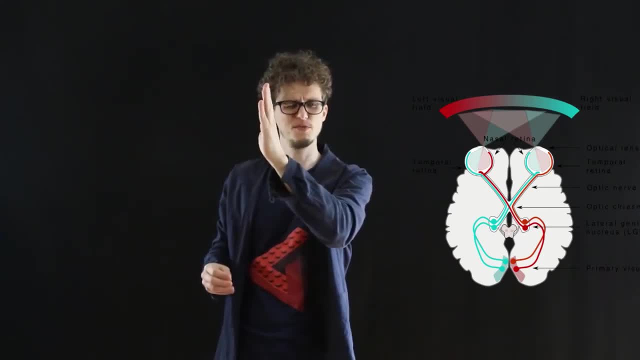 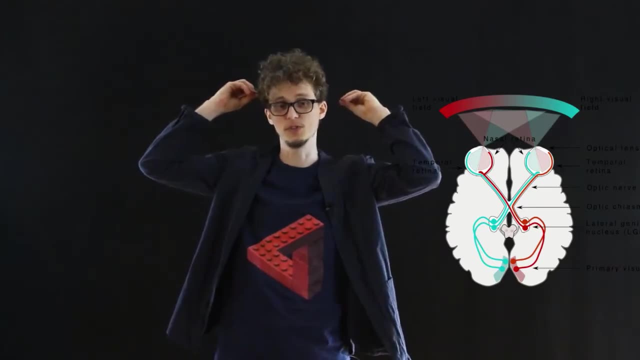 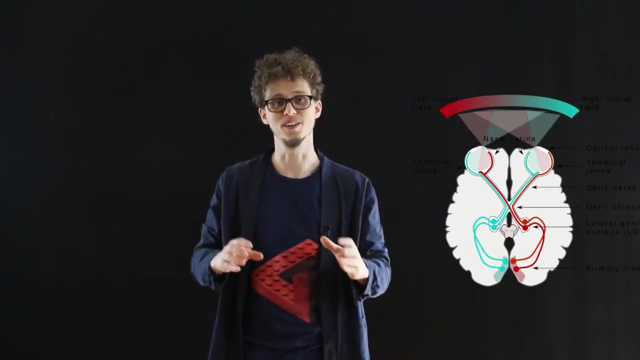 It travels along a pathway to the right hemisphere, and your right visual field travels along a pathway that's processed by your left hemisphere. And only after each of those streams goes to V1, to your occipital lobe in the back of your head, only then do they get recombined at a later point, after they've already been. 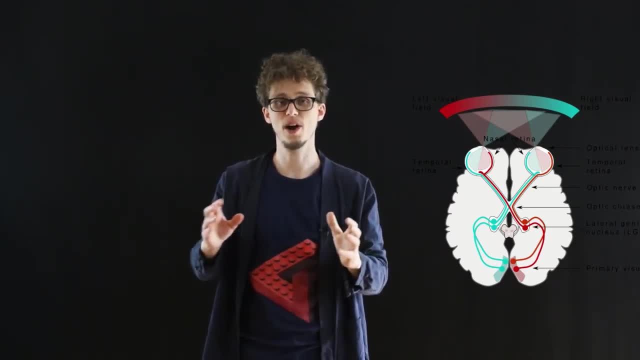 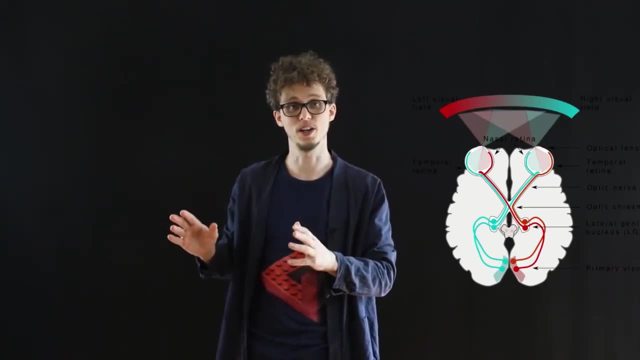 initially processed, This might not seem that wacky, but it's going to have some pretty wacky effects that we're going to talk about in the future when we talk about neuroscience and when we talk about split brain patients. So sensation is the act of taking that information from the outside world, transducing it into 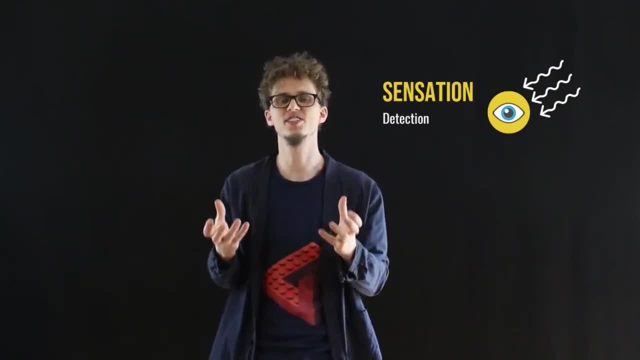 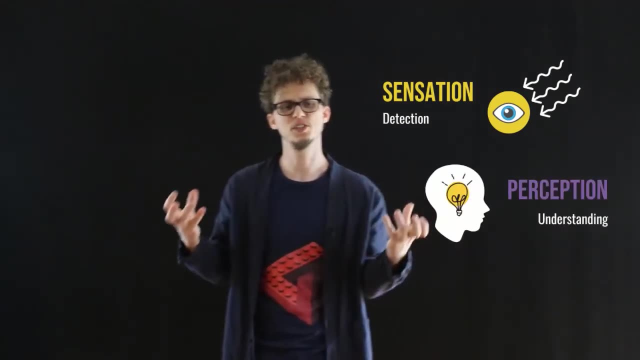 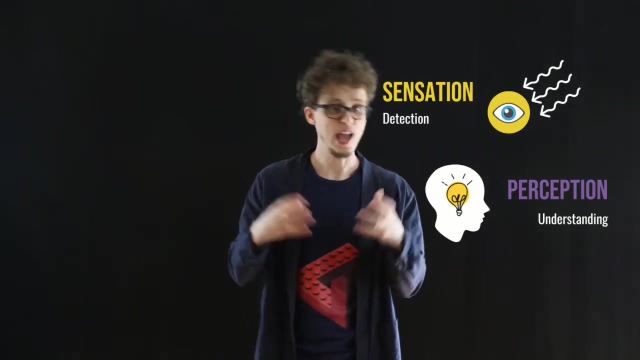 a format that our brains can comprehend, Just taking and detecting information. But perception is a much more complex process. Perception is a process of taking that information and building it into something meaningful to us, interpreting it, generating some kind of understanding about the outside world. 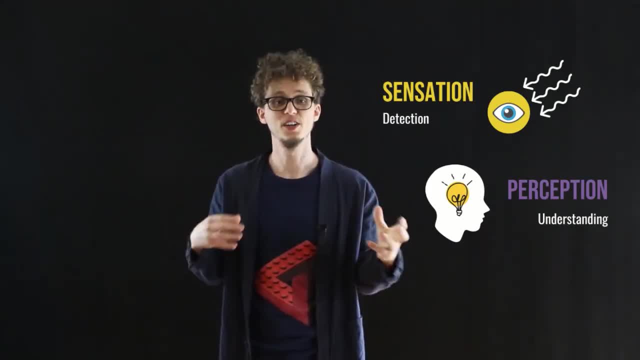 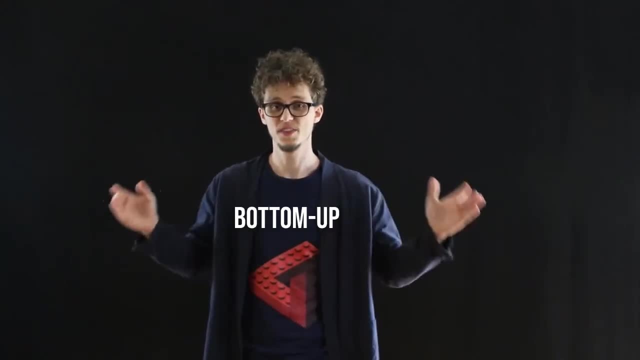 And this process, the perceptual process, can go in two directions. We can build representations, We can build representations of things in the outside world from the bottom up, taking that information from our sense organs and just building a representation out of whatever information is available. 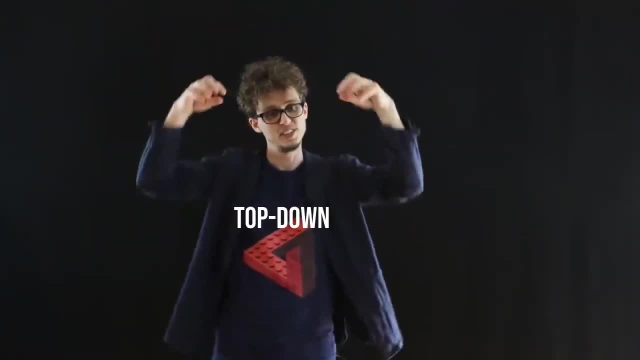 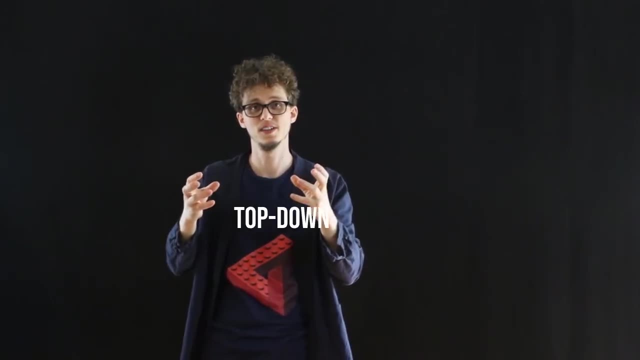 But we can also build representations from the top down, taking what we already know about the world and using that to influence the type of representation that we generate. So we can think about this system as being a sort of hypothesis generating and hypothesis testing mechanism. 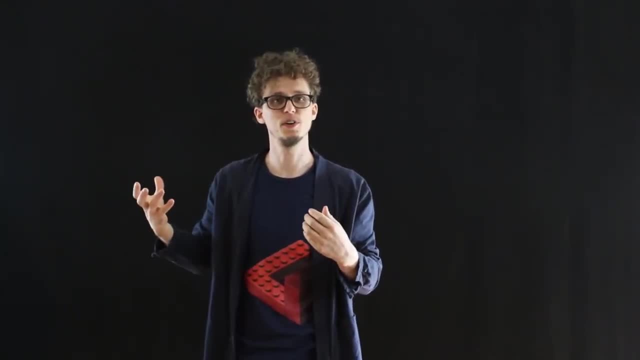 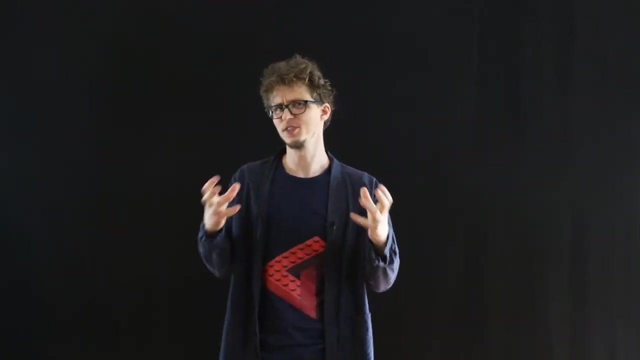 We have conceptual knowledge about the world- knowledge that we gain from experience- and we use that knowledge to influence the type of representation that we are creating. the model of the world that we create- Perception- involves lots of top down processes. We make lots of assumptions about the world and we use what we know about the world to 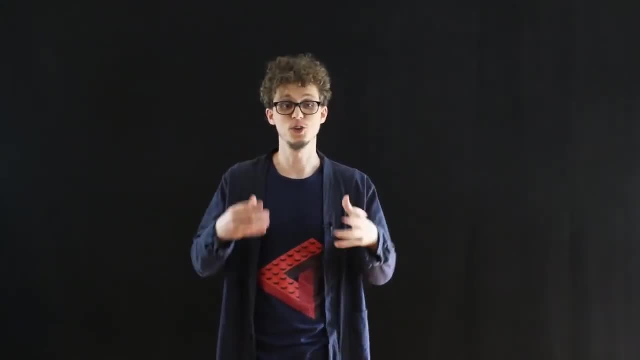 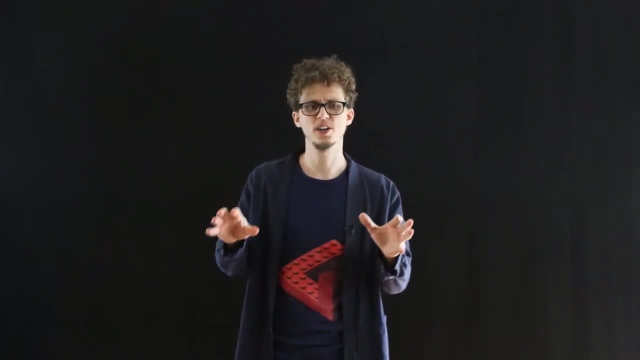 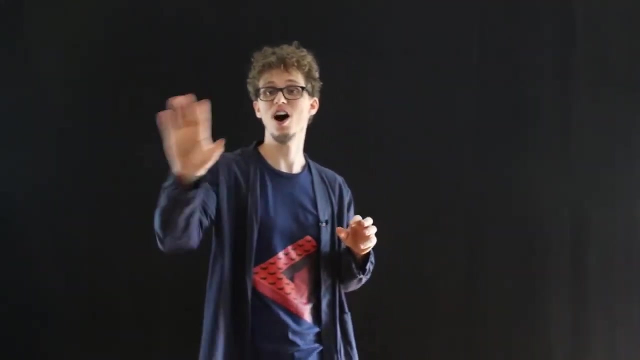 update our perception of the things that we are seeing so that they make sense, Because, really, what our minds care about when we are trying to navigate the world, we don't care necessarily about the physical status of the light entering our body. What we really care about is the physical status of the objects in the world that are 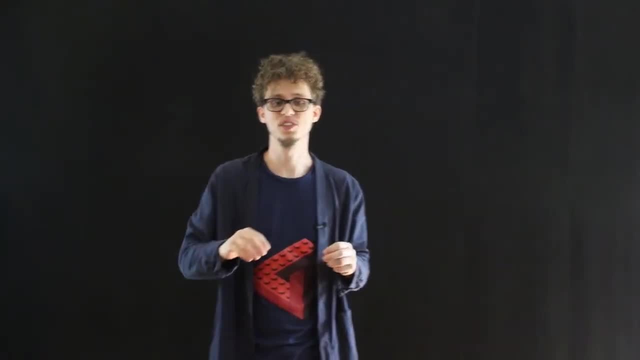 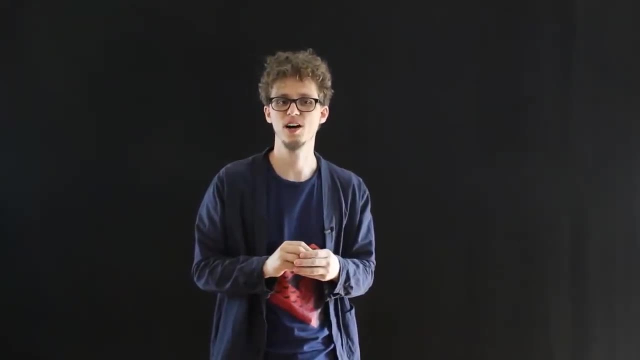 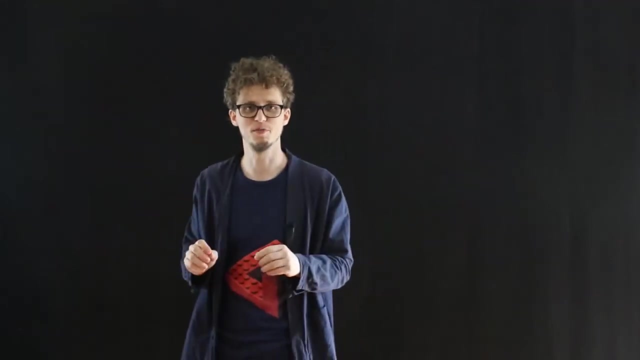 reflecting the light. So we make assumptions to try to recreate an accurate representation of that thing in the world that the light is reflecting off of. It's not the light that matters. It's what we think the light can tell us about the thing that it's bouncing off of. 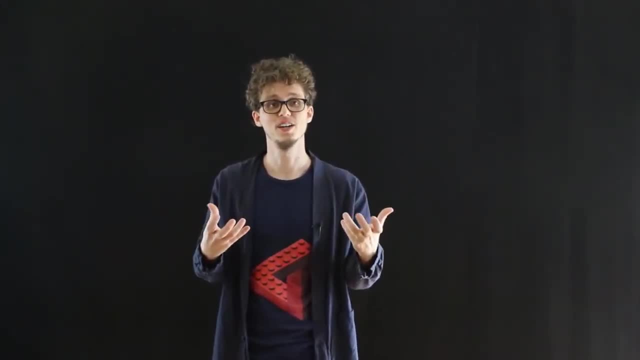 So our mind does lots of interesting things. It might make an assumption like the fact that an object's color. It might make an assumption like the fact that an object's color. It might make an assumption like the fact that an object's color doesn't change just. 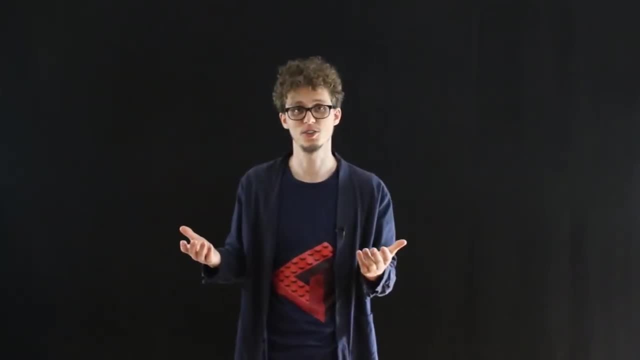 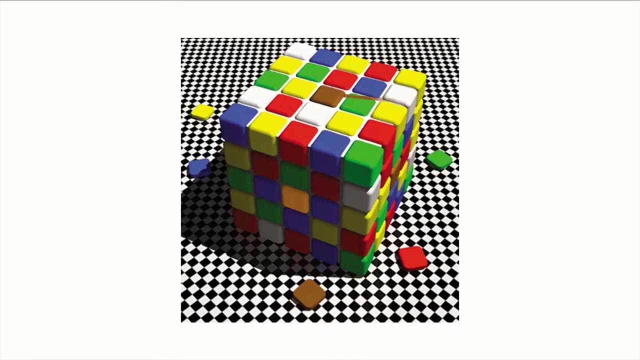 because the color of the light that it is bathed in has changed. Take an example like this cube with lots of colored squares. On one face it has a square that looks very brown. On another face you can see a similar square that looks very orange. 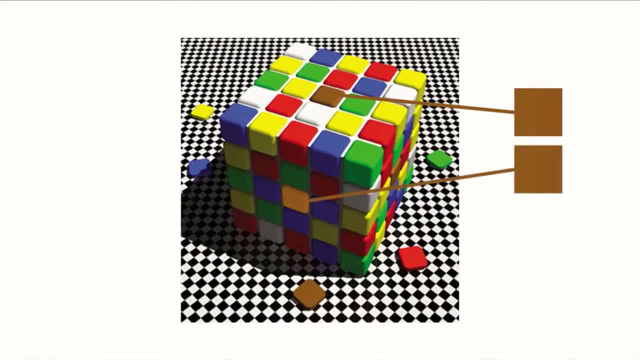 If we sample the color from both of those quadrants, we can see that actually, they are in fact an identical color in terms of the raw input. The light that is entering our eyes is the same, But we don't perceive it as the same. 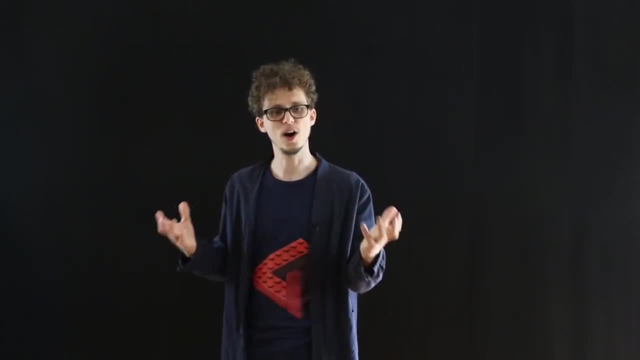 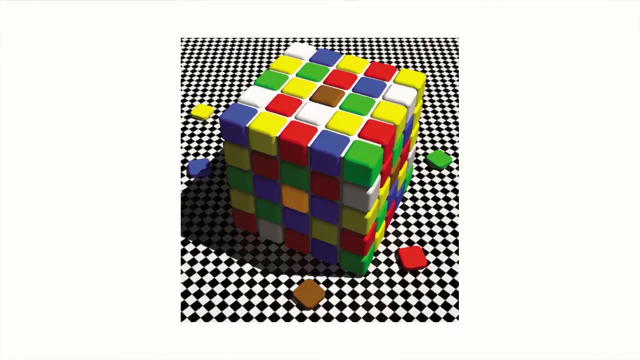 We perceive two very different colors. Why? Why is that? Well, one of those faces is in bright light, The other face is in shadow, And what our mind is trying to do is trying to recreate what we think those underlying colors actually are. 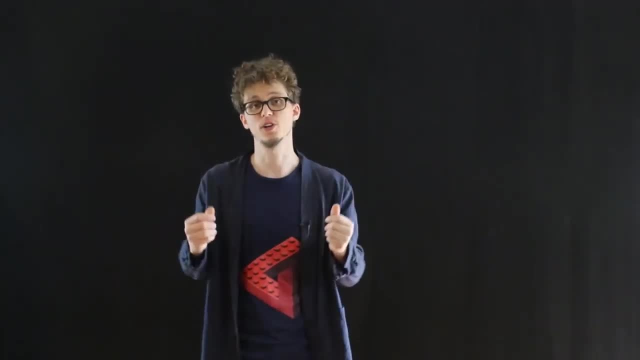 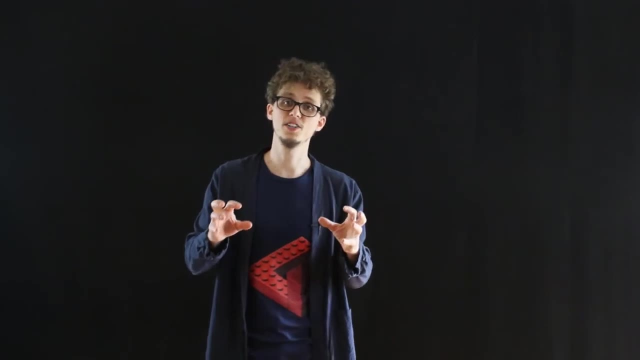 The specific value of the color that we're actually seeing, of the light that's entering our eyes, is less important to the mind than what we think the color of the actual light is. So, in a sense, what our mind is doing is it's sort of subtracting out the effect of the 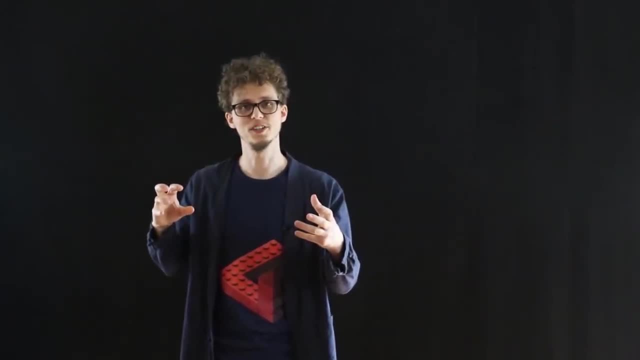 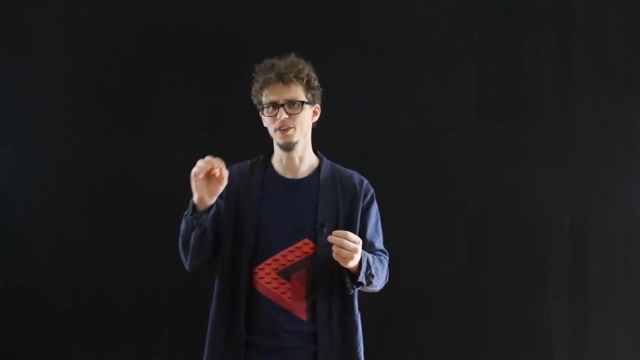 shadow. It's performing some kind of correction And it's that process, that corrective process, that makes one of those colors look like orange and the other look like brown, even though they're actually physically the same color. We can take this a step further. 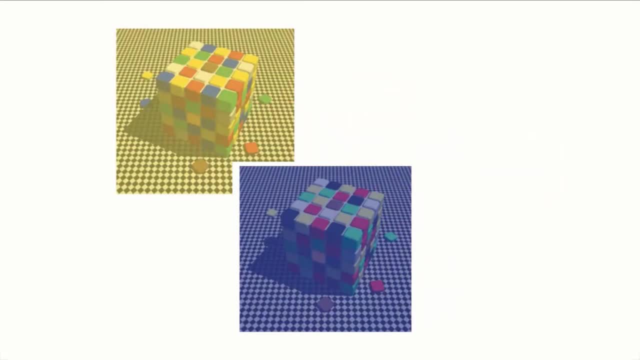 We can bathe the image of the cube in yellow light and then sample a color which looks very much like blue. Then we can take the cube and we can bathe it in blue light And we can take a sample of a color that looks very much like yellow. 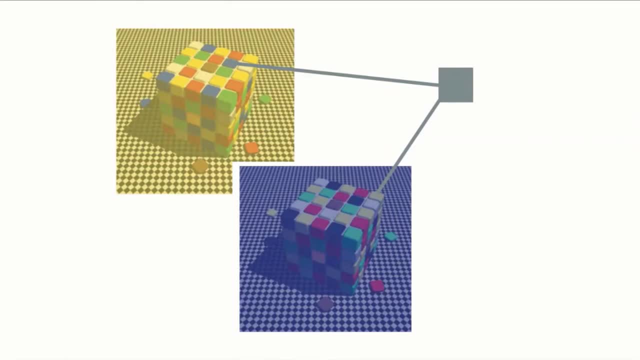 And when we sample both of those squares, what we find is they are actually physically identical. They are identical color values in terms of the raw light. The raw input going into our eyes is the same, And yet we have an incredibly different experience of those two colors. 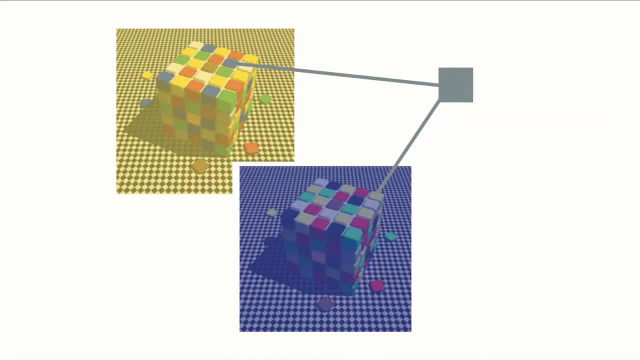 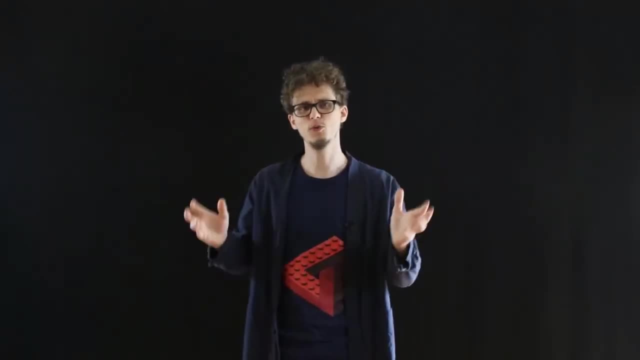 One of them looks extremely different, The other one looks extremely different. The other one looks extremely blue, The other looks extremely yellow. So how is it that in fact, they are actually both gray? How can that be? How can we perceive them as yellow and blue when in fact they are both just gray? 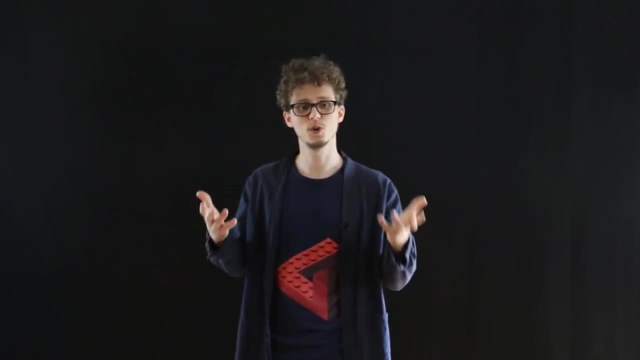 Well, it's the same process. We are correcting for a sort of color imbalance. We see that the image is bathed in yellow light, And so we are shifting our perception of that gray cube towards blue, away from yellow, And vice versa. 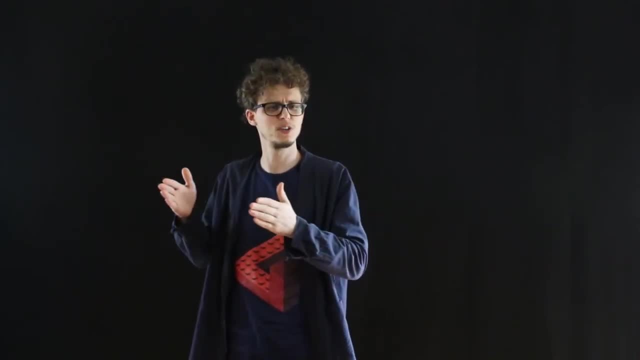 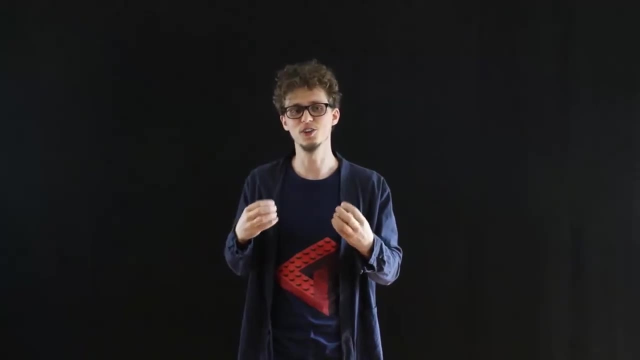 When it's bathed in blue light, we are shifting it away from gray, towards yellow, away from blue. This is all our mind's sophisticated way of trying to understand the ground-level reality in the world, by removing these extraneous environmental artifacts, removing color keeping. 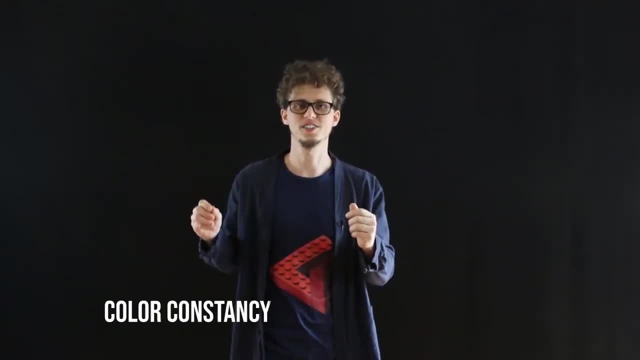 things constant. This is called color constancy, sometimes referred to as color constancy illusions. What our brain cares about is not what color is. It cares about the color. It cares about the color it's actually seeing, not what color is hitting the rods and cones. 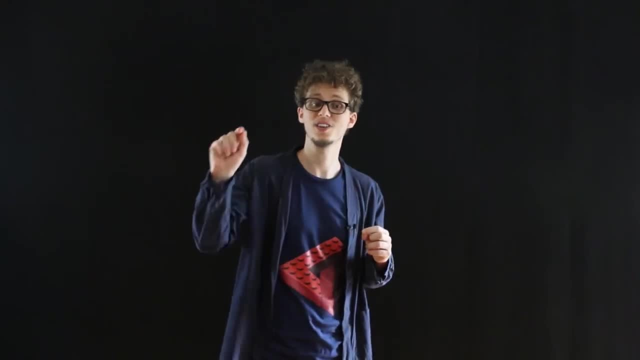 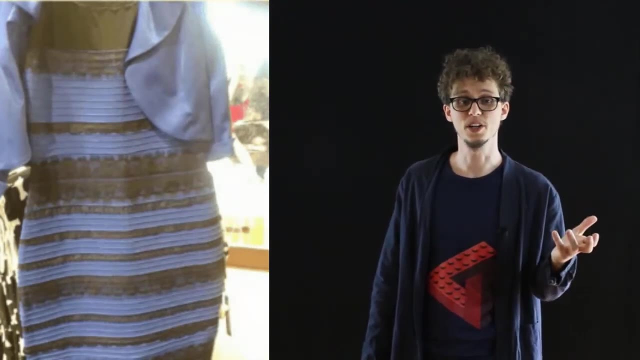 in our eyes. What we care about is what color we think that object actually is. Here's another example that you probably remember. That's right. I'm bringing this back, All of those horrible memories. I'm reopening all of these wounds. 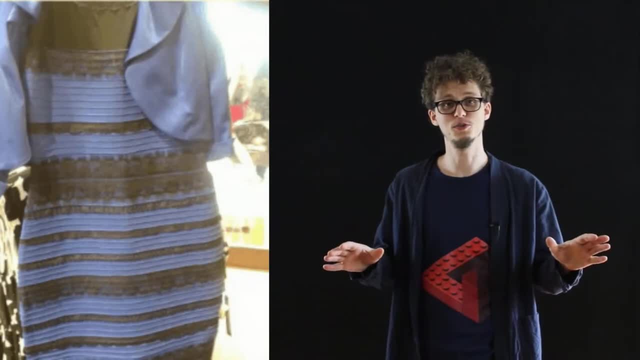 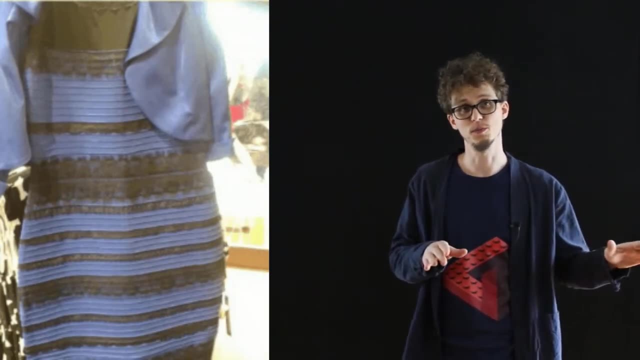 That's right. it's the dress. Now I'm not going to ask you what you see it as, because I don't want to start some kind of war. We'll just say that some people view this dress very strongly as being blue. 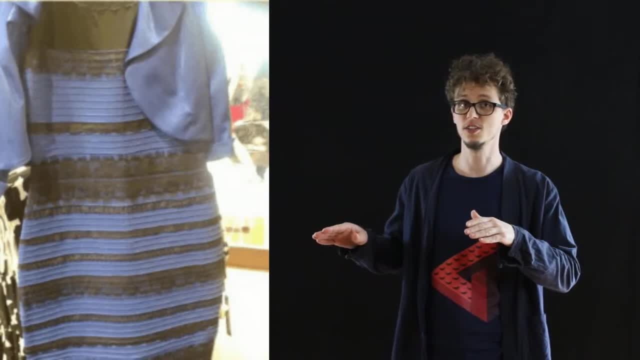 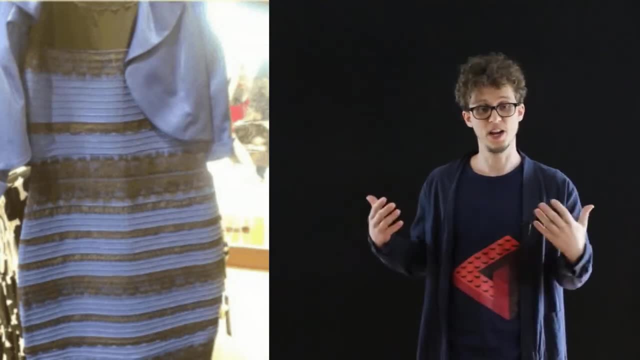 And some people have a very strong intuition that the dress is white and gold. I'll put my own reputation on the line here and say I am one of those people that sees white and gold And I know that it's wrong. I know that now. 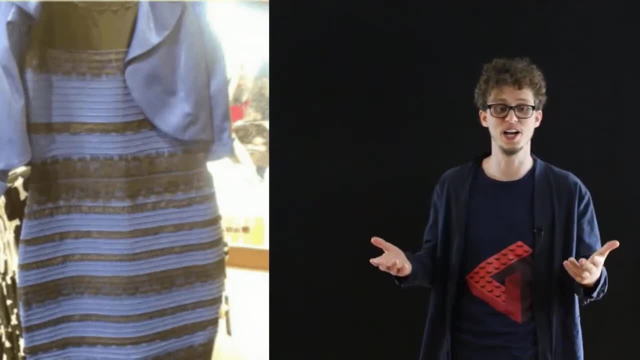 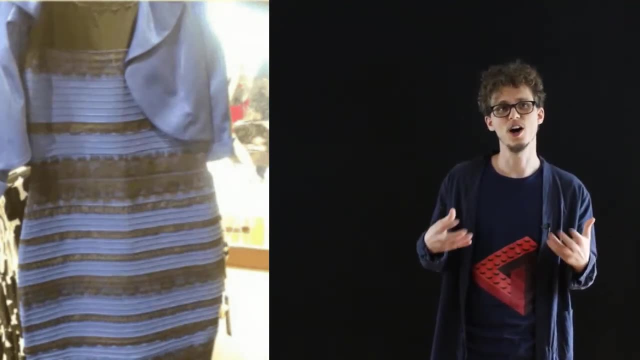 I've seen the corrected images and I know what color the dress actually is in real life. So this is actually kind of a problem. I've been saying that what our brains are trying to do is to reconstruct the underlying colors that the object actually is. 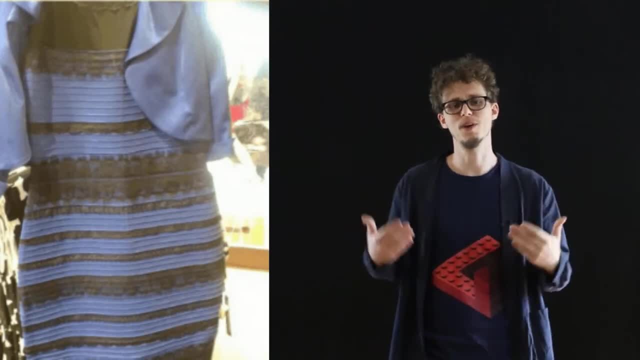 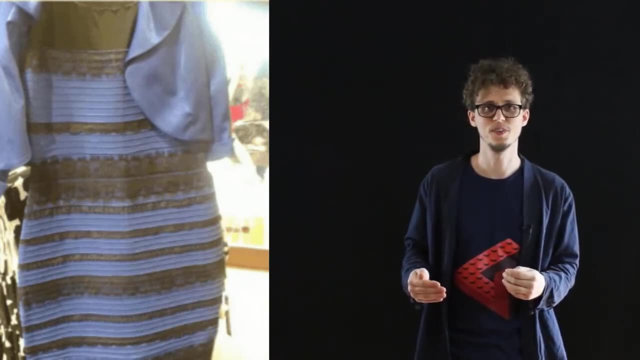 So how could I be so wrong? What's going wrong in my mind that's causing me to get the wrong percept? I'm reconstructing the wrong underlying color. Well, it has to do with what kind of assumptions we're making about what we think the lighting 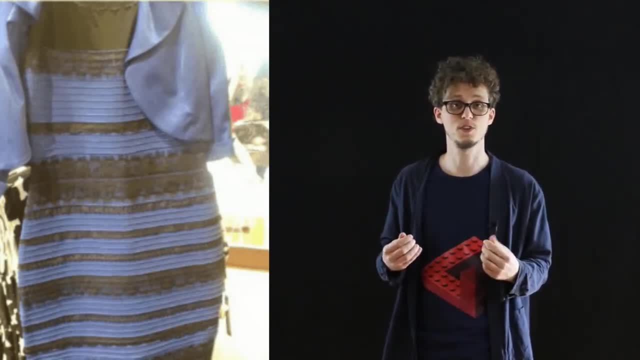 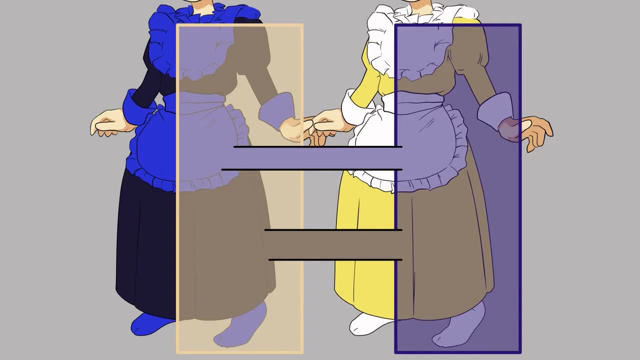 conditions are. Remember that our brain is correcting for these different kinds of lighting conditions. We're trying to figure out what the actual color of the thing is supposed to be. Well, if you assume that what you're seeing is a blue and black object under harsh yellow, 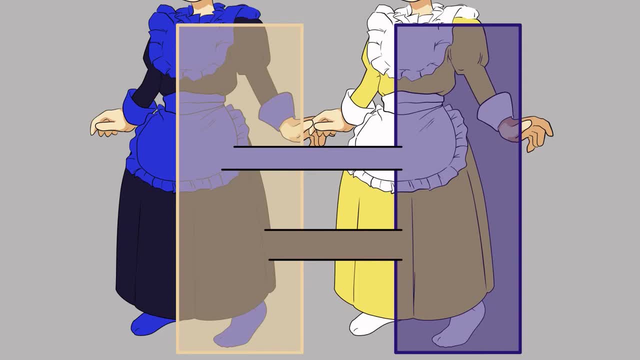 light. Well then, that makes perfect sense That it looks like this. Your brain can do a correction to subtract some of the yellow light, push it in the direction of blue. But if you assume that actually what you're viewing is something that's under a shadow, 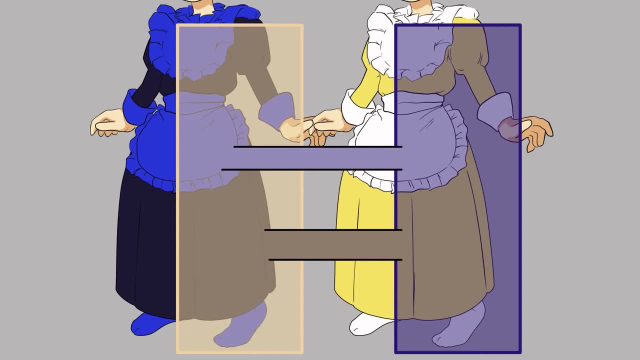 I see bright illumination in the background. Maybe this is something where it's like outdoors, but it's under a tree, or something like that. Well then, I might make a correction in the other direction. I might shift it away from blue towards yellow. 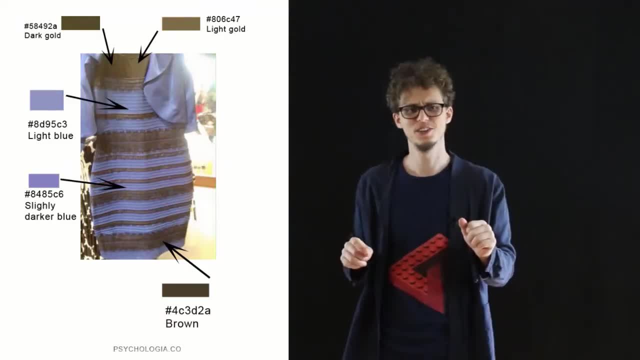 Of course, if we actually sample those colors, we see that There isn't actually white or gold and there isn't really a blue or black. What we really get is kind of a muddy brown and a kind of a light desaturated blue. 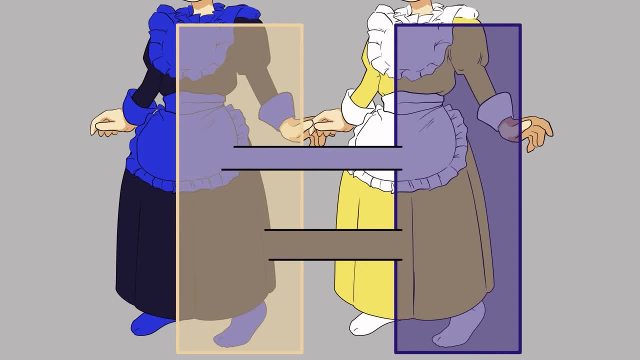 Turns out, you can view these colors either as that dark, rich blue and black, or as a white and a yellow, depending on what kind of lighting conditions you think are present. So our perceptual system is making lots of assumptions about the underlying reality of the thing that we're witnessing. 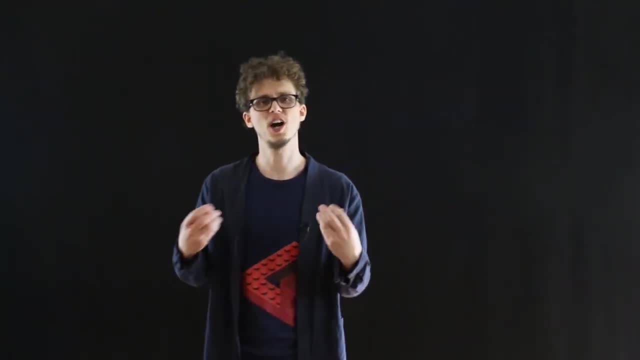 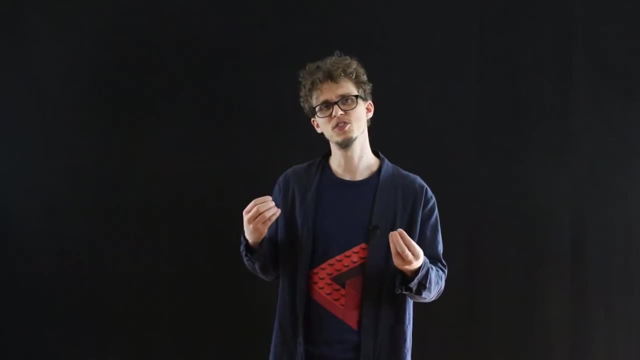 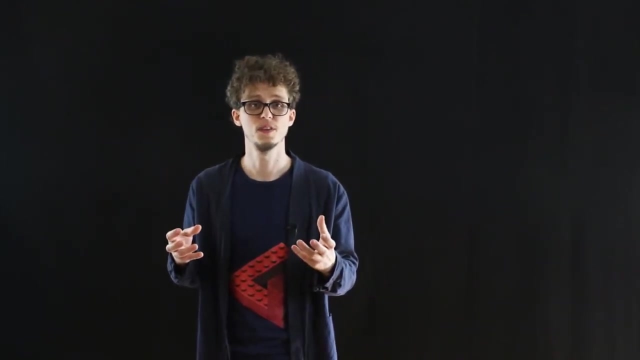 It makes assumptions about color. It makes an assumption that color doesn't change, that color is invariant even when light is changing. Our minds also make assumptions about the constitution of objects, that objects should be whole even if their parts are covered. So if I show you an image like this, it just seems to be a bunch of shattered stuff, just. 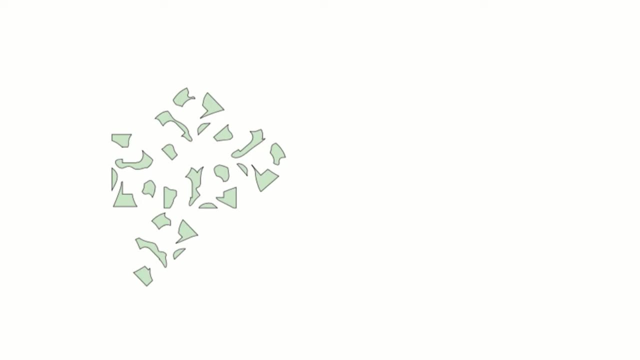 remnants of something garbage, Who knows. It doesn't look like anything in particular, But if we put a very strategic inkblot Covering all of those empty spaces, suddenly it becomes very clear what this is. Our brains can now complete the image. 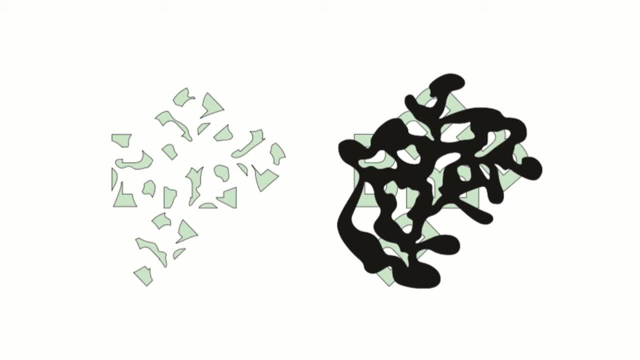 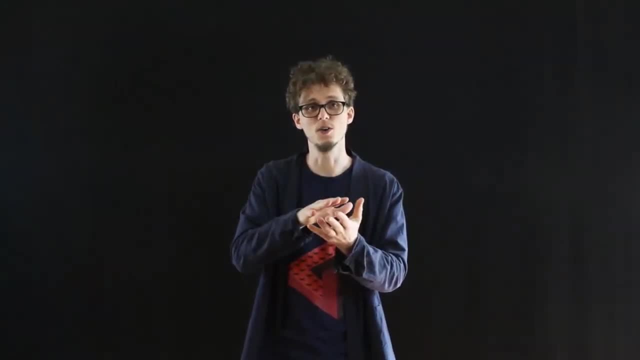 Oh, it's a whole bunch of letter B's underneath some obscuring ink. The addition of that ink gives our brain valuable information. It says: oh, that's actually not empty space. There's something under here that we should be reconstructing. 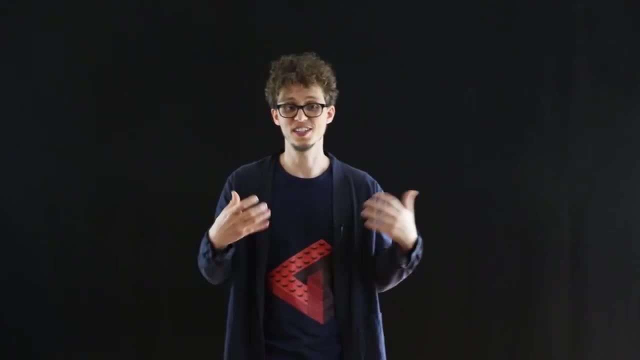 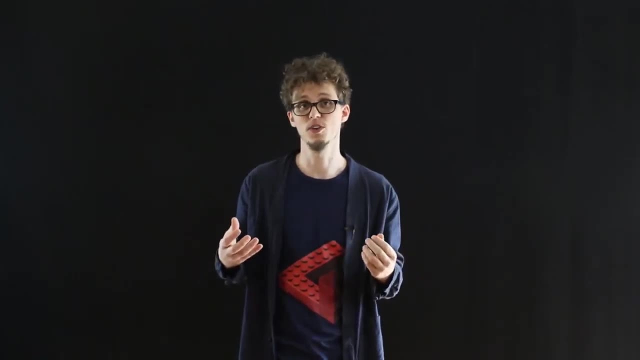 And it turns out to be quite easy to reconstruct that once we know that that's a valid assumption that we can make That there is something, That there is something That there is something to be reconstructed. So this is a very active process that our brains do all the time. 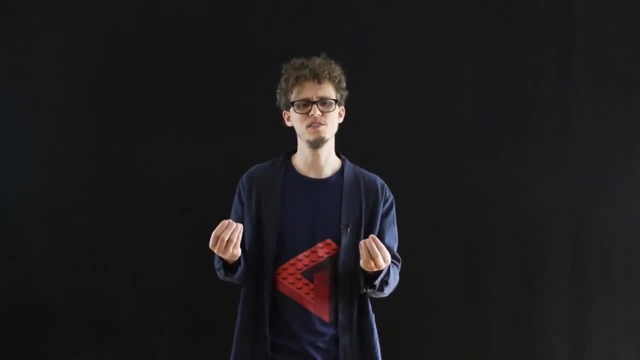 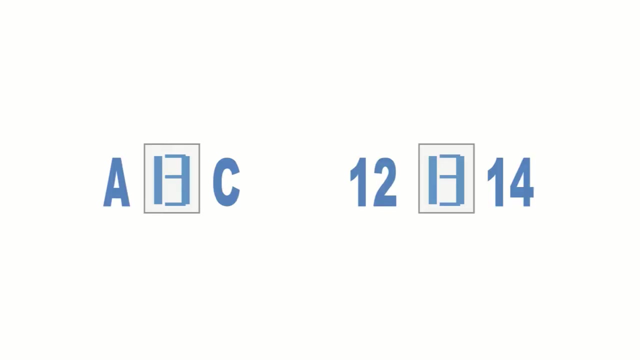 This is referred to as amodal completion: being able to complete figures and objects if they are partially obscured. So that's an example of our minds using knowledge about the world to fill in missing information. Here's another example. This is an example in which our minds will resolve an ambiguity by using what we know. 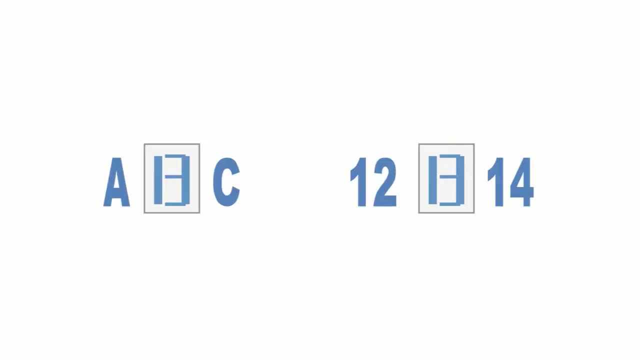 about the world to fill in missing information. Notice here that the same shape is recognized as a different symbol in each context, Either a, B or a 13. So the same shape can be recognized as either a letter or a number. It's ambiguous. 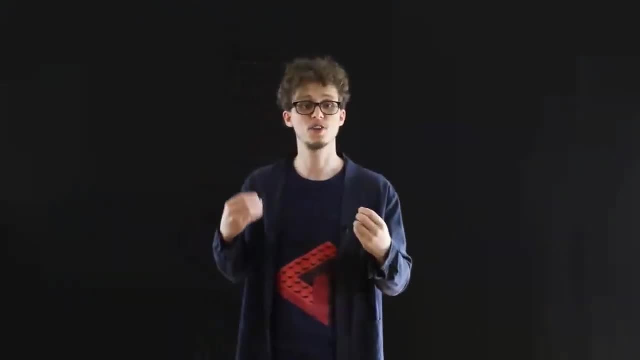 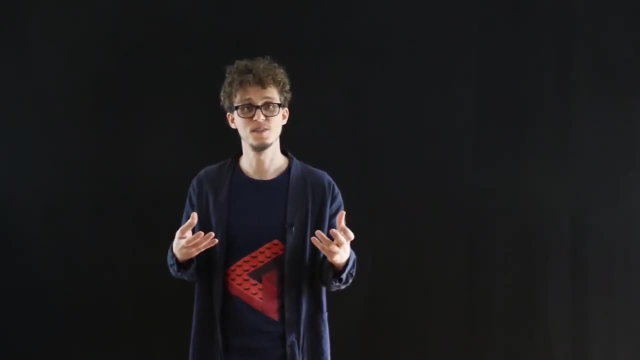 So this is another piece of evidence that our minds are doing an awful lot of top-down processing. We are using what we know about the world to fill in gaps and missing information. We're very good at this. We're very good at filling in missing information and resolving ambiguity and making predictions. 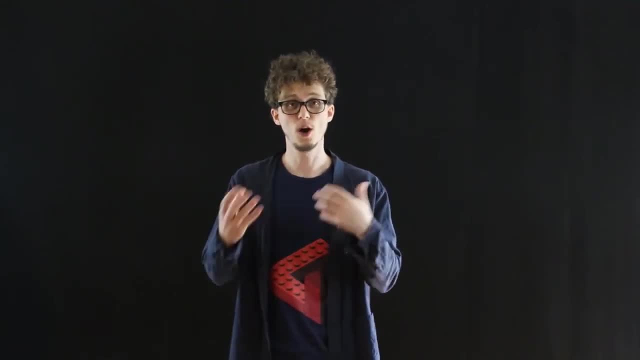 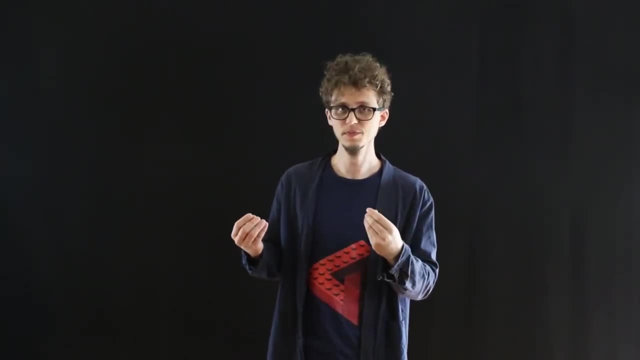 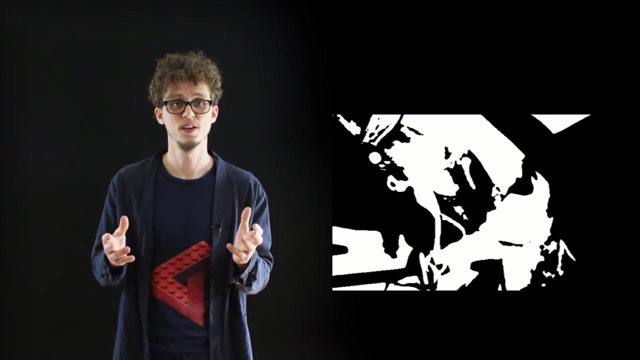 What we perceive also relies on attention. Where we choose to focus our gaze, or what we choose to focus on, can affect what we perceive. Here's an image that may not seem very meaningful. In fact, it may not look like anything in particular. 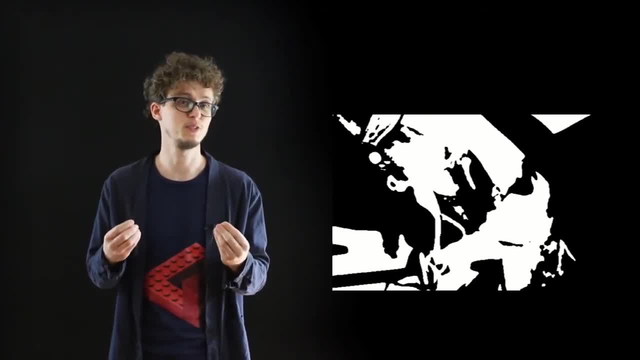 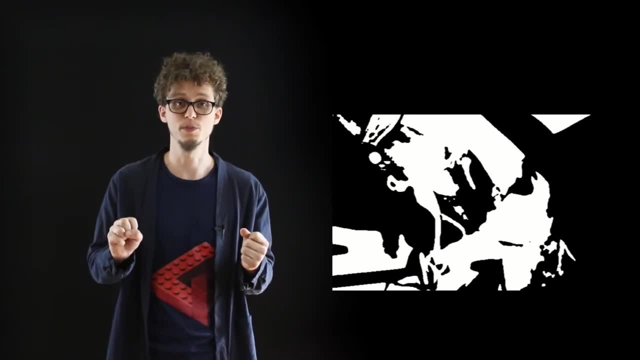 That's because we don't have quite enough information to reconstruct what this was supposed to be an image of. It just looks like some vague dark shapes. But if we fill in that information, I show you what the original image was. Oh, so it's just an image. 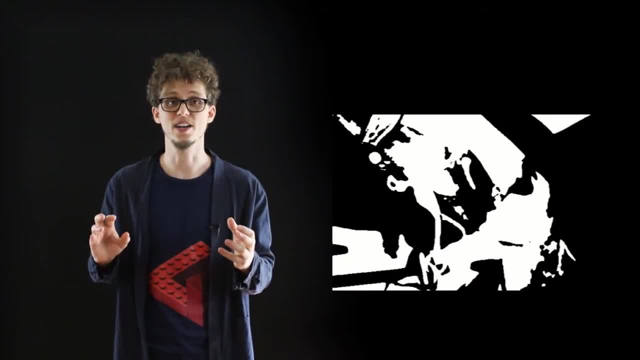 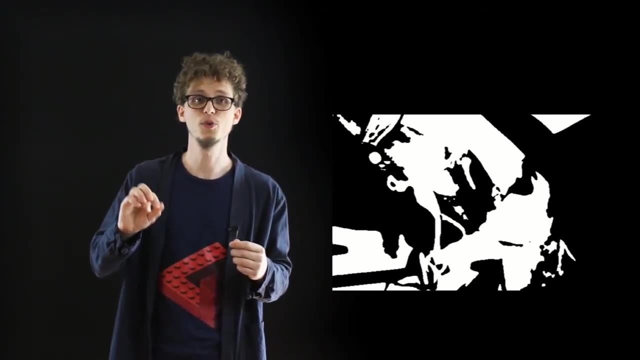 Oh, it suddenly becomes very obvious. And now, if I take that away and I see the original image again, now I can't help but see the original image, I can't help but reconstruct what this image was actually meant to be. So once we have that information about what this thing is, we can reconstruct it easily. 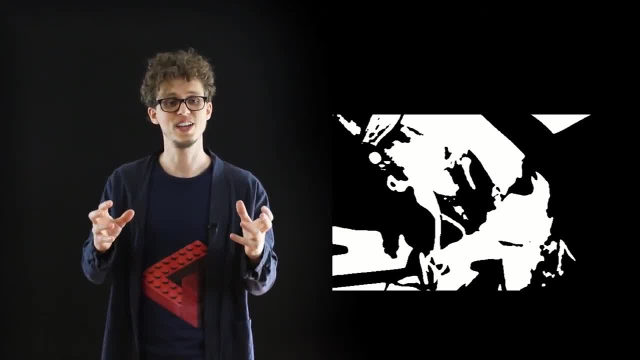 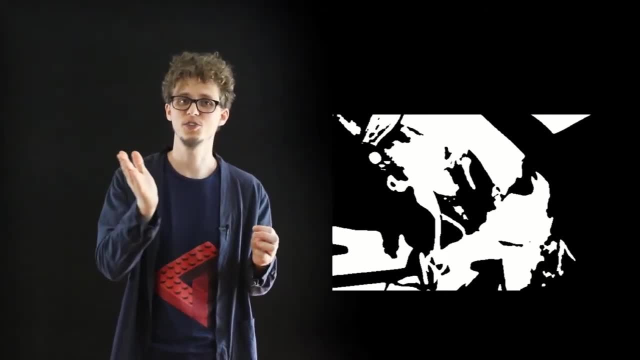 from even just a small amount of information. Why is that? It's because we are now attending to the right parts of the image. Now we know that some of these mysterious inkblots are actually the boundary of a world. Now we know that some of these mysterious inkblots are actually the boundary of a world. 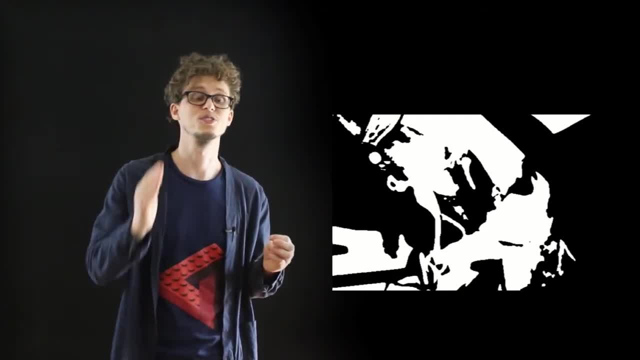 Now we know that some of these mysterious inkblots are actually the boundary of a world. Now we know that some of these mysterious inkblots are actually the boundary of a face or the boundary of the horse's nose. We're able to draw those outlines in the right places because we are attending to the right. 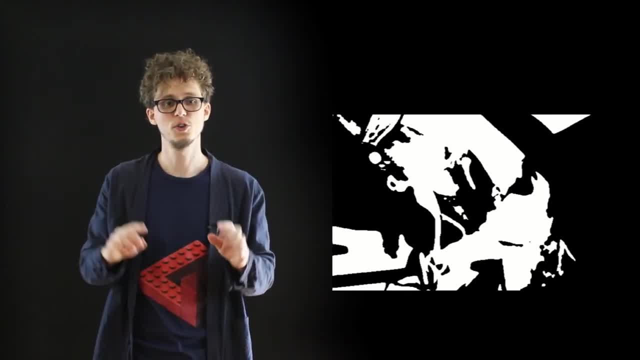 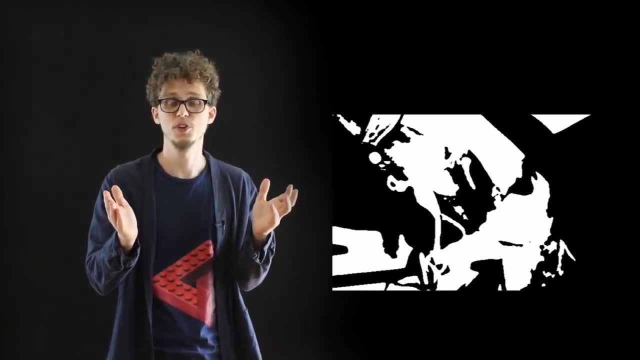 areas of the image. So there are two elements at play here. There's the role of attention, figuring out what parts of the image we should be focusing on, But there's also the role of memory. Once we know, once we have that world knowledge, we can use that to fill in those missing pieces. 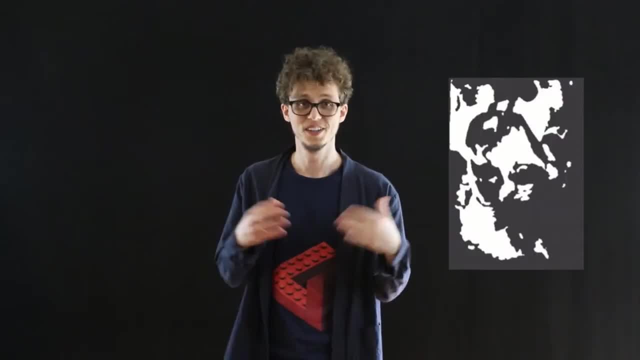 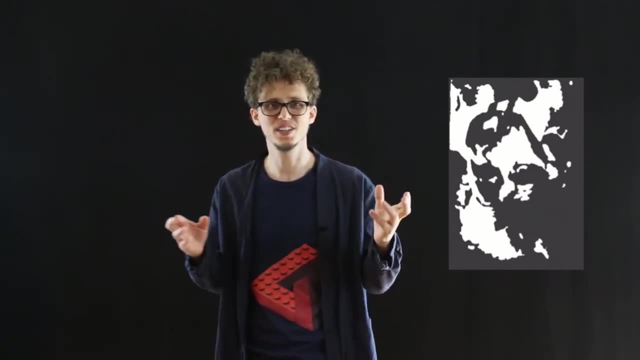 to fill in the gaps. Here's another example. This is another very minimal image. It's just inkblots on paper and it might not look like anything. Maybe you can kind of see a face or something. Is it a recognizable person? 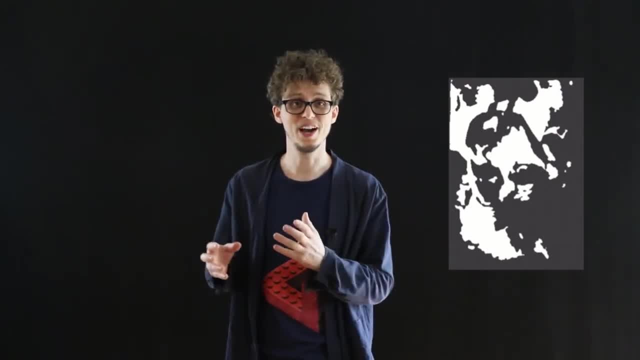 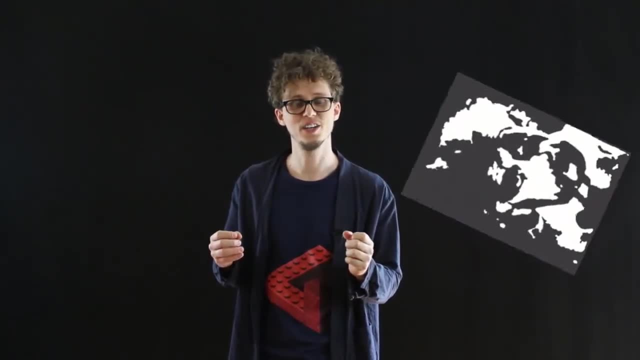 Can you tell who this is supposed to be a portrait of? Maybe not. It probably looks kind of chaotic and messy. It might not look like anything in particular, But if we rotate it 180 degrees does it suddenly come into focus. Who is this? 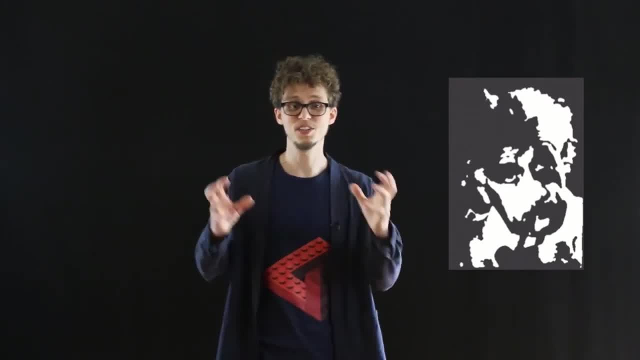 It's a very famous person. It's Albert Einstein. It probably seems a lot clearer now that it's right side up. So again, the way in which we perceive the image relies a lot on what we're paying attention to. When the image is upside down, we can't quite figure out what features we should attend. 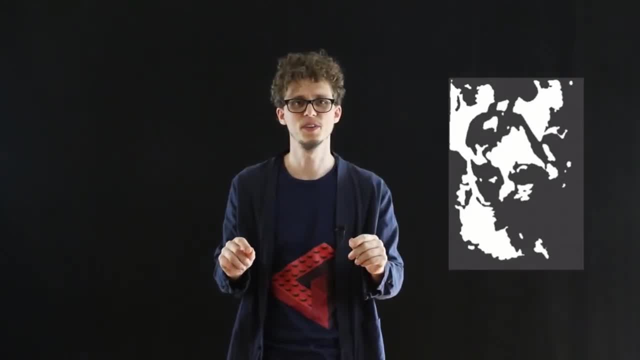 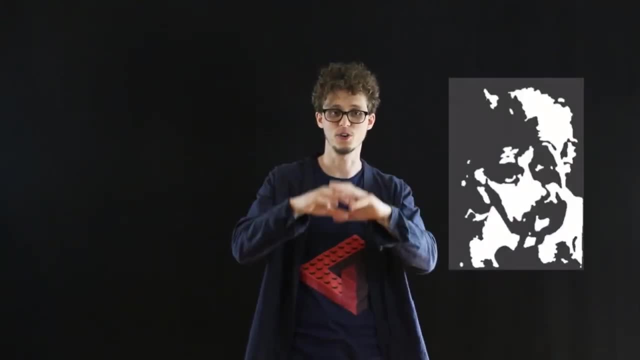 to Our eyes sort of skip over the image almost at random, Flipped over right way around. now it becomes very clear: There are eyes and a mouth, And now I know what to focus on in order to recreate this image. Recognizing faces is actually a very difficult thing to do. 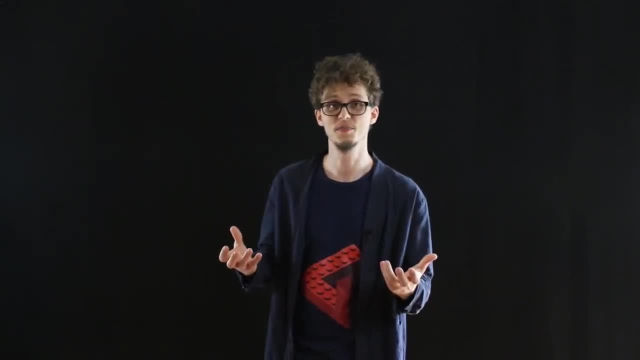 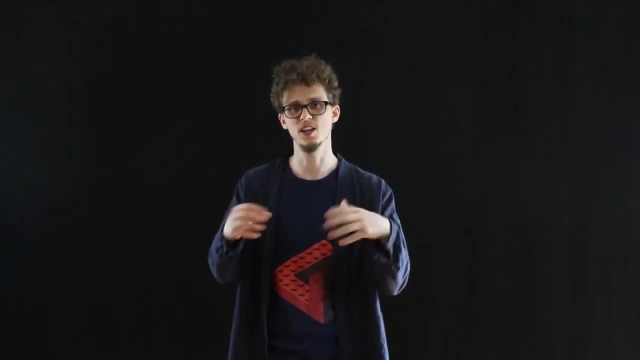 That we mostly take for granted. It's sort of an automatic and inherent part of our perceptual system to be able to take all of those features of human face and immediately map it to a person that we know. But not everyone has that ability. 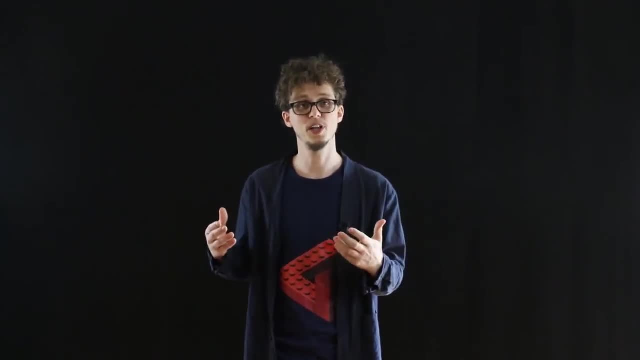 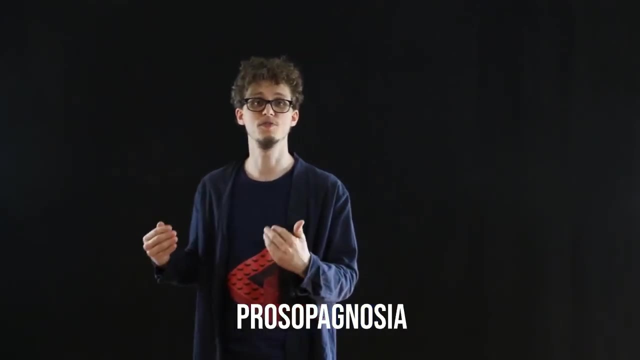 We may take it for granted, but there are people- about 2% of the population- that are face blind. They have prosopagnosia, an inability to recognize human faces, And that's not just a big thing, It's a big thing. 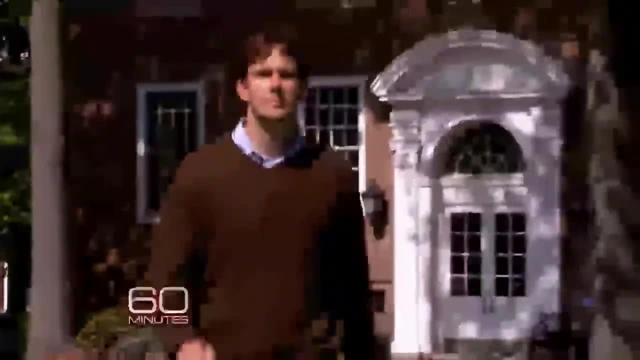 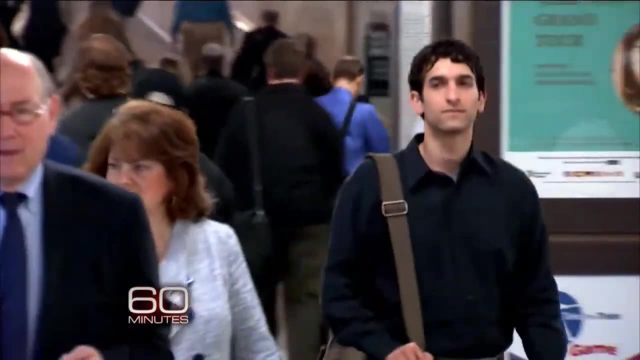 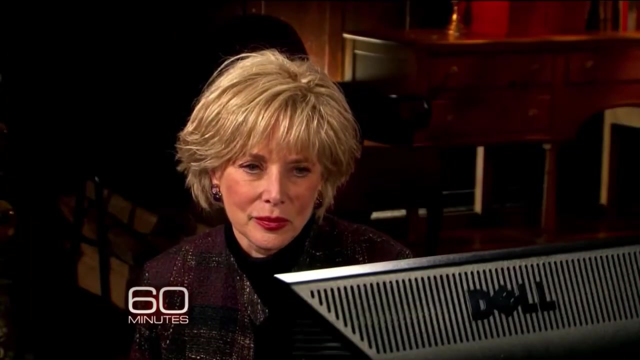 It's a big thing, is a professor at Dartmouth College who's been studying face blindness for nearly 15 years. He says the hardest thing to understand is how people can see a familiar face but not recognize it. So he created a demonstration to give me a little taste. Faces turned upside down. 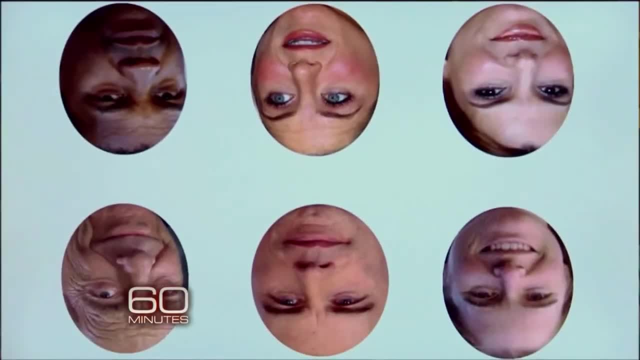 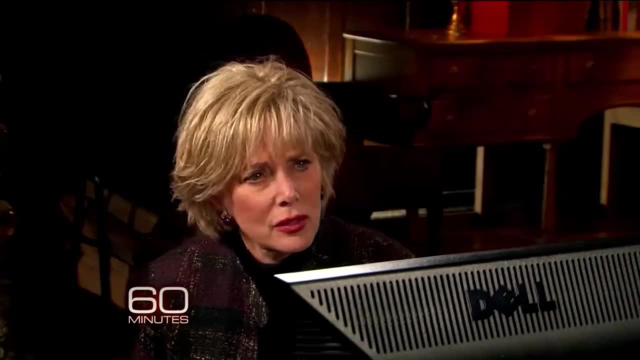 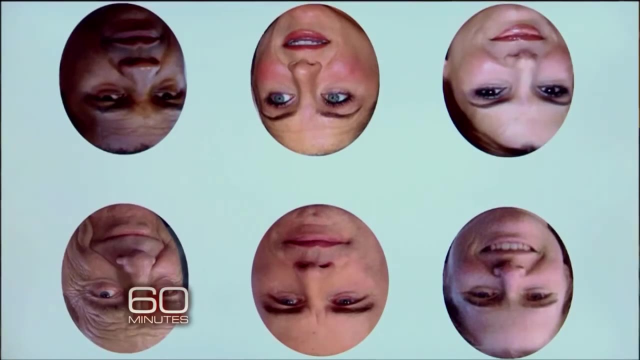 So here are some famous faces. You're going to be tempted to twist your head, but don't do it. Okay, Can you identify any of these people? I was completely at a loss. You think I'd know all of these people. You've seen them all a lot. I don't know any of these people. I really don't. 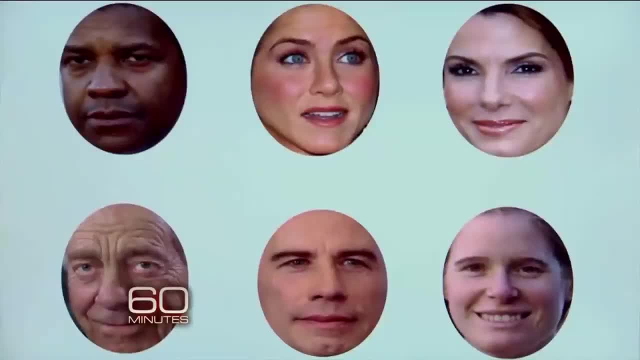 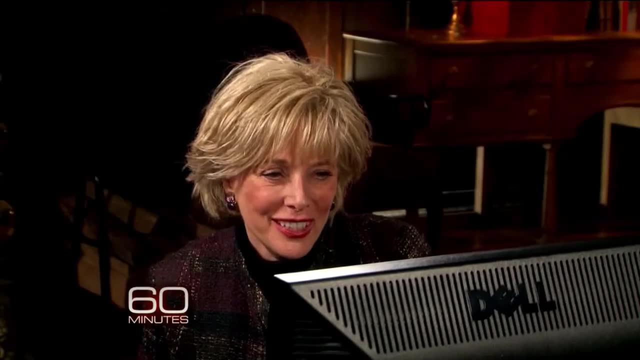 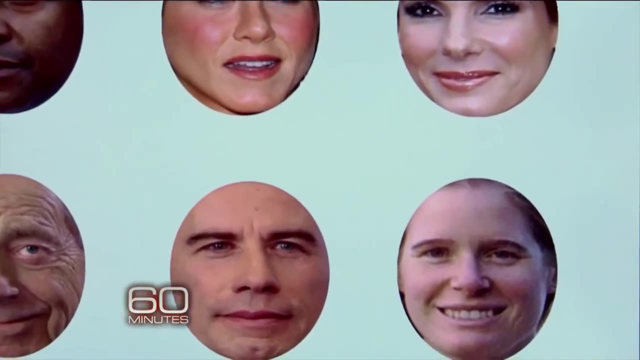 Do you want to see them upright? Sure, It was astonishing. With just that click, they became recognizable people before my eyes. I know John Travolta, I know Morley, And there was Denzel Washington, Jennifer Aniston, Sandra Bullock, But the one that really got me was the young woman on the 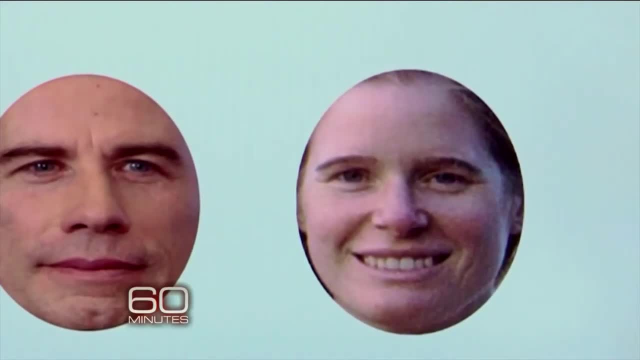 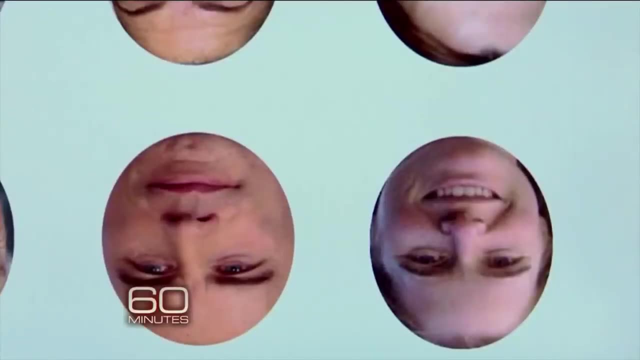 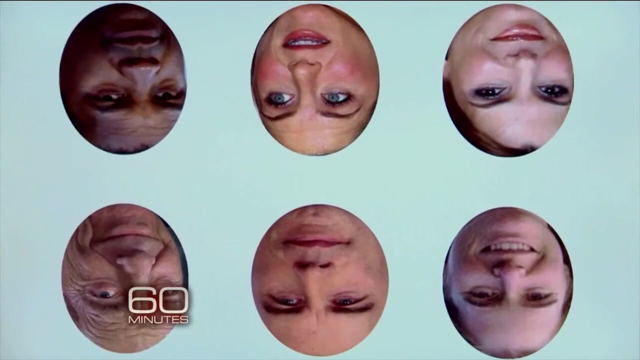 lower right, my daughter. I didn't know my own daughter. No, I didn't know my own daughter, So there she is. Wow, So is this? am I getting a feeling for what people with face blindness have? This is when you look at that. there's clearly, there's a face there. Oh yeah, There are parts. 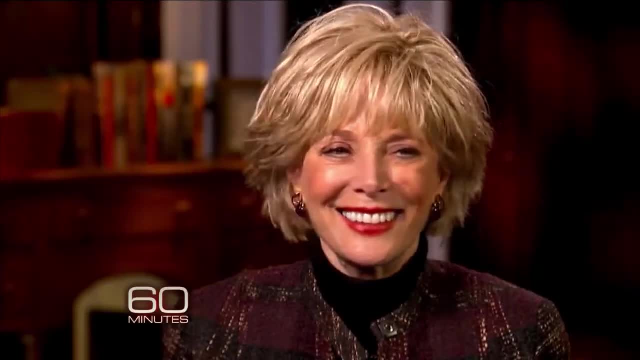 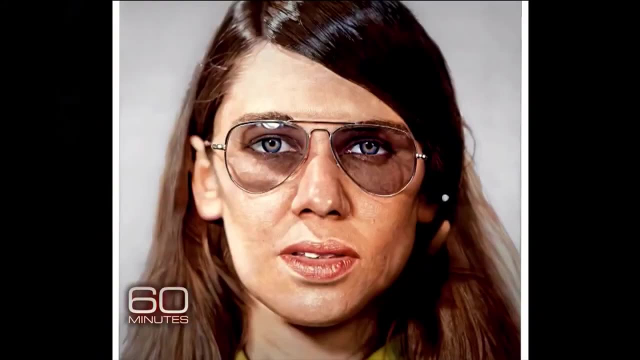 there are eyes, there's mouth, but you just can't put it together. Wow. Faces have captivated artists forever, So it may surprise you to learn that the man who painted these faces, renowned portraitist Chuck Close, is also face blind, and severely so. 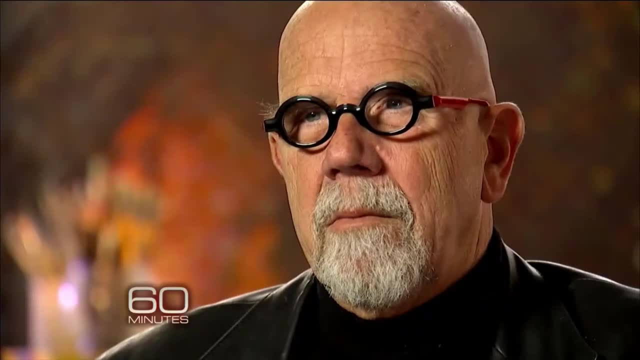 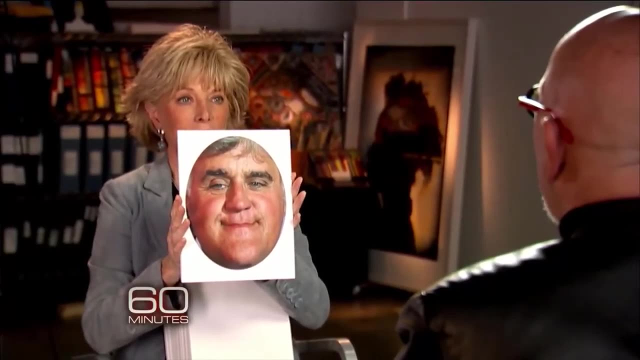 Let's say you went out to have dinner with somebody and then you saw her the next day, Wouldn't remember her. We brought some of our famous faces along to show him From the chin- I think it's Leno- And we're surprised that he did pretty darn well. 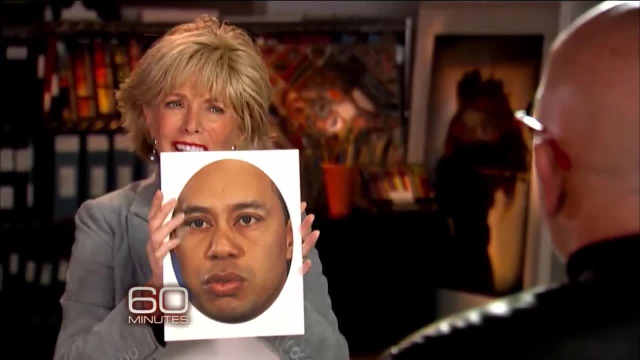 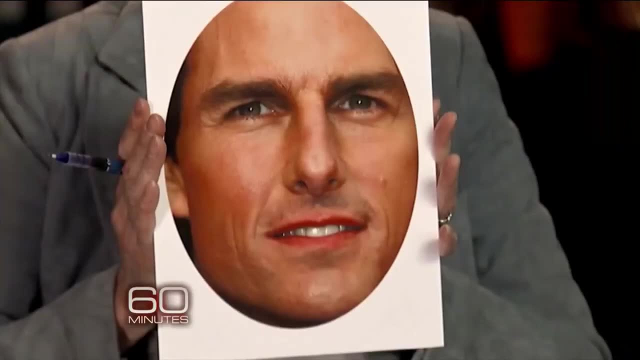 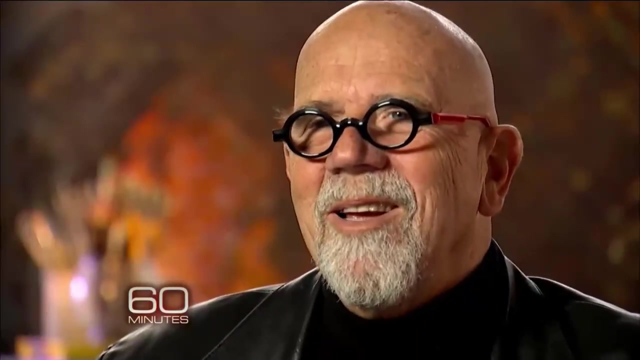 Well, from the lips, I think it's. I think it's Tiger Woods. Yeah Well, you're pretty good, But of course not perfect. I don't have a clue. That's Tom Cruise. Right now, my guts are tied in knots because this very activity is the thing that makes me most nervous. 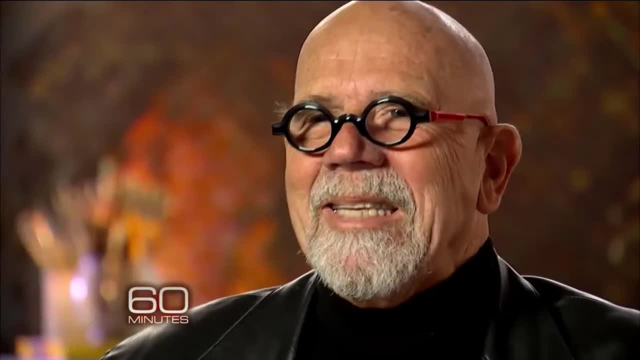 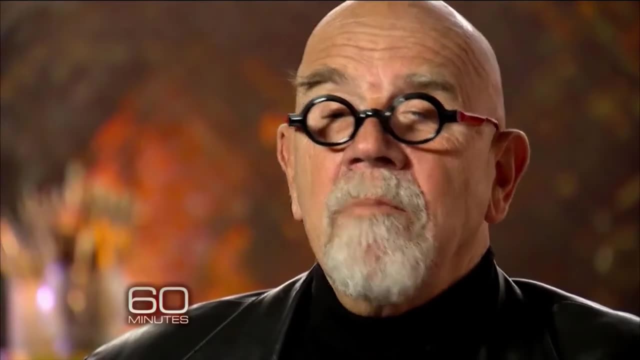 Oh, now I have to figure out who this person is, Because he isn't recognizing these faces the way most of us do. Every face is a puzzle he has to solve What I'm thinking? you don't see too many people with just a mustache anymore. 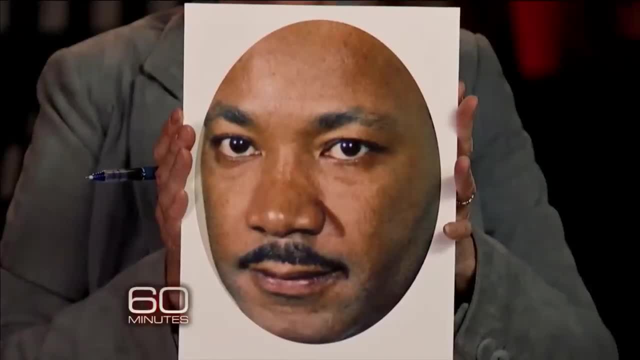 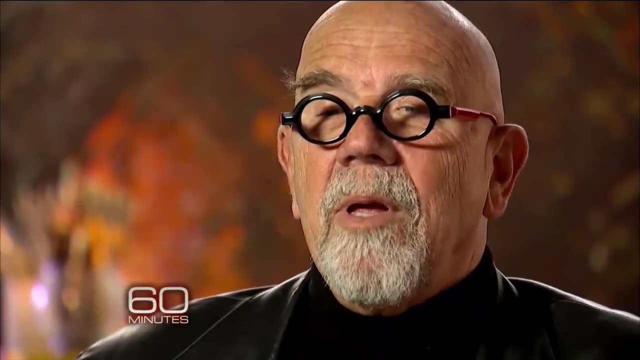 So that means it's probably somebody who's not alive. So if it's an African-American of a certain age with a mustache, it might be Martin Luther King. You're amazing: You deduce, deduce, deduce. You're like Sherlock Holmes here. 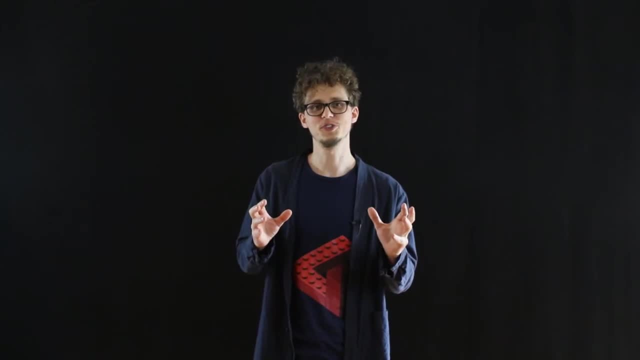 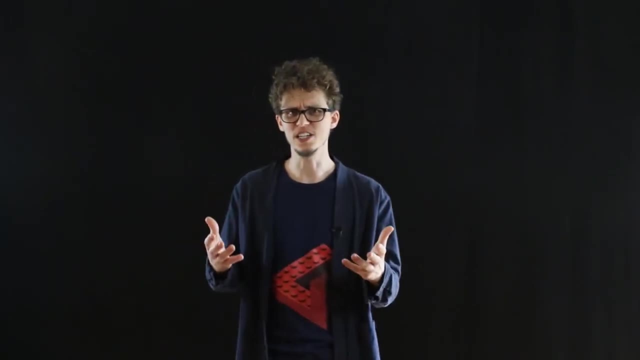 This is how I get through life. Face blindness is interesting because it illustrates the difference between sensation and perception. People with face blindness don't have any trouble seeing human faces. They can see you fine. There's nothing wrong with their visual system. 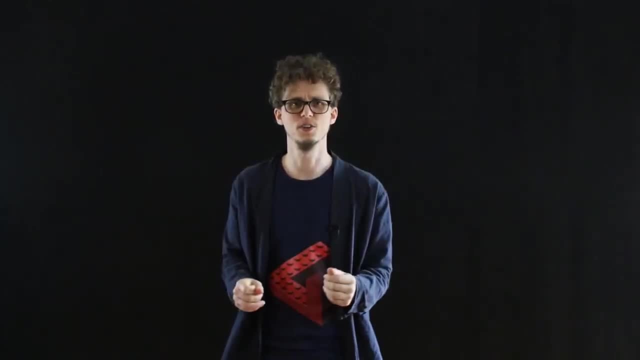 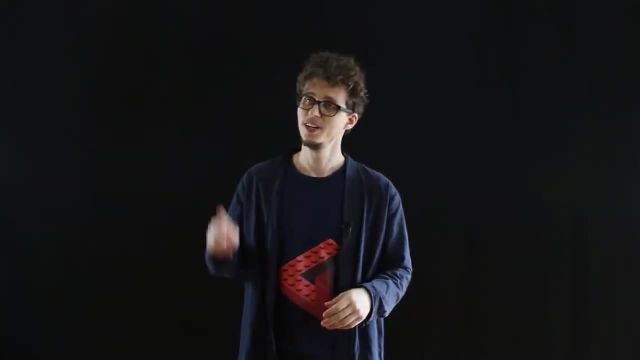 They can make sense of the fact that you have two eyes and a nose and a mouth. They don't have any problem seeing it, But they do have some impaired perception. There's another condition that I think highlights the difference between sensation and perception. 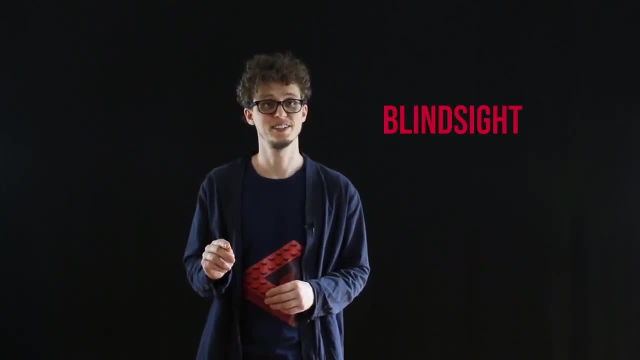 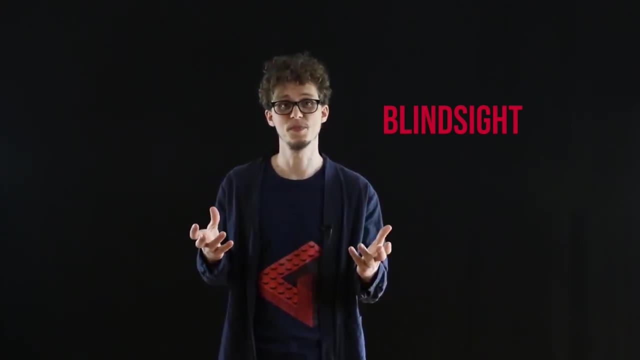 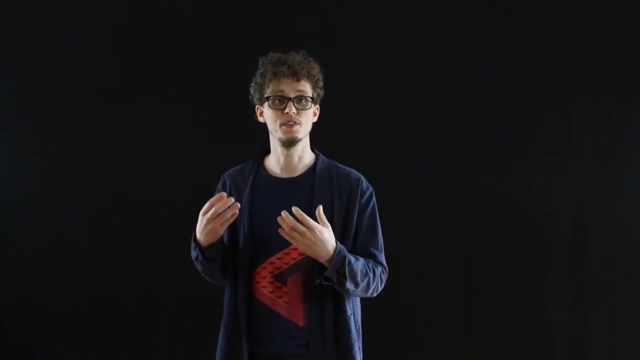 And that condition is called blindsight. Blindsight is a kind of blindness. It results in people being blind, Not being able to see, But rather than there being something wrong with their eyes, blindsight is caused when there is something wrong with the visual cortex. 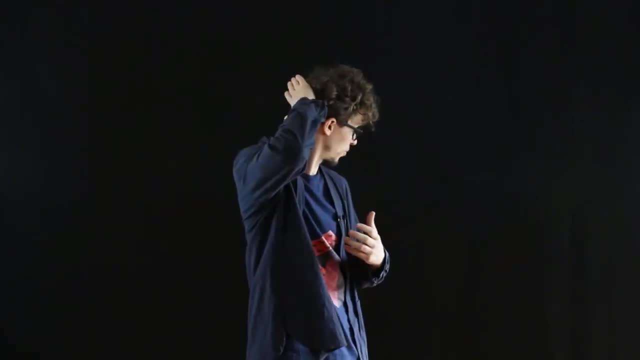 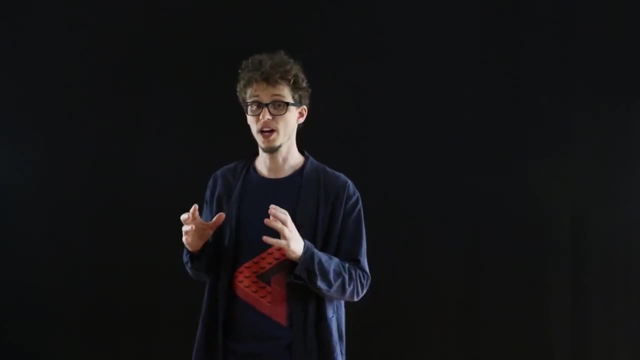 For example, if you've had a certain kind of brain damage, Damage to this part of your brain, the occipital lobe. The interesting thing about blindsight is that people with blindsight, although they are blind, they cannot see things in their environment. 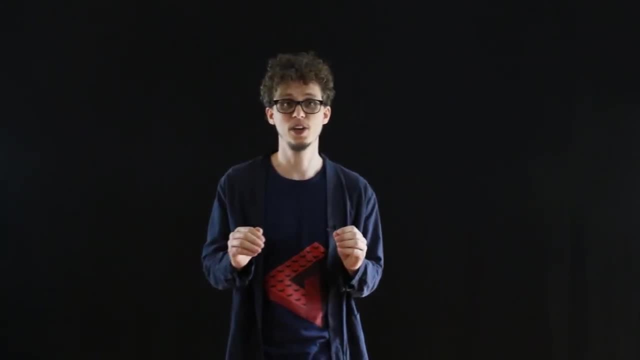 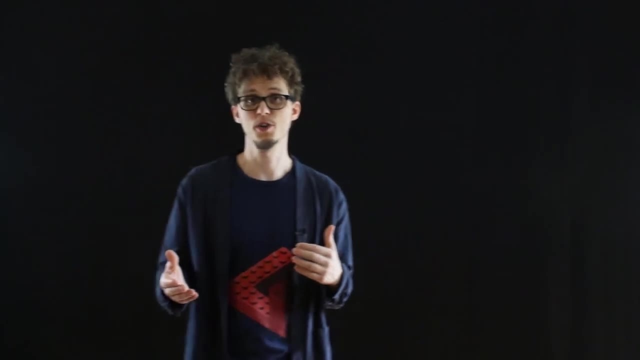 They do have some ability to detect motion and location. There have been lots of experiments Performed on people with blindsight, Where a researcher will show them something on a screen Like horizontal lines, And they'll say: Tell me what's on the screen. 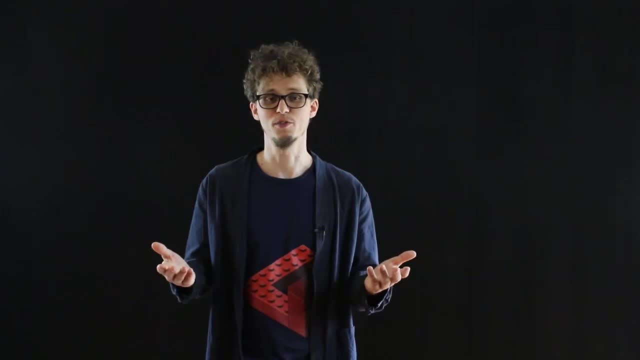 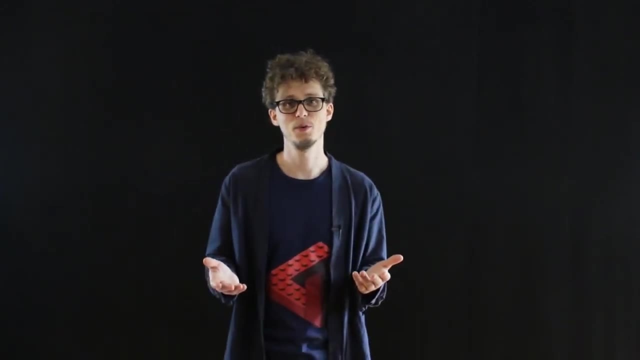 And the person with blindsight says, Uh, I'm blind, I have no idea what you're talking about. And he says, Well, why don't you just guess? And they say, Well, I guess, I see, maybe some like horizontal stripes. 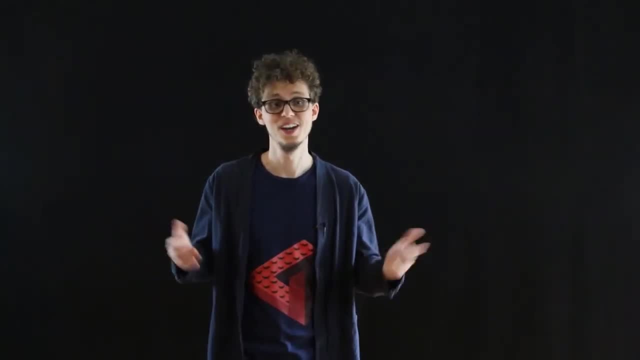 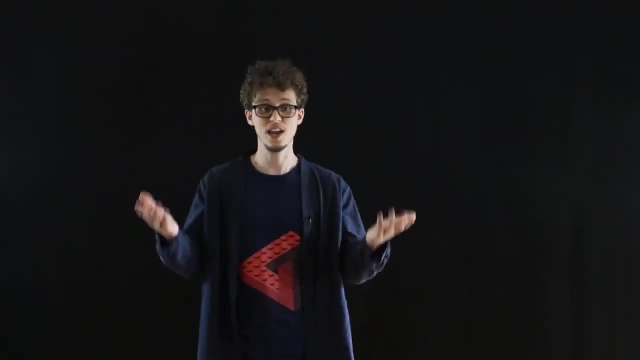 I guess I have no way of knowing because I don't actually see anything. But the crazy part is that they are often right Their guesses, which they're making totally blindly right. They have no idea what they're looking at on the screen. 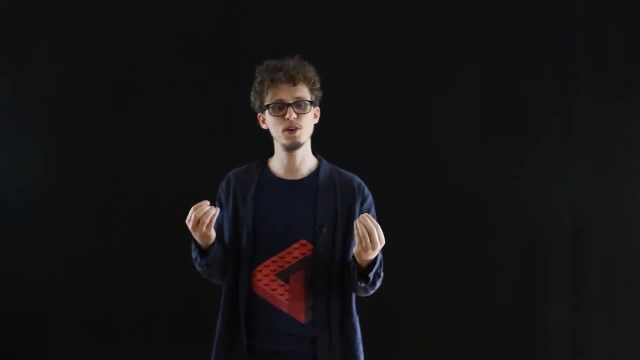 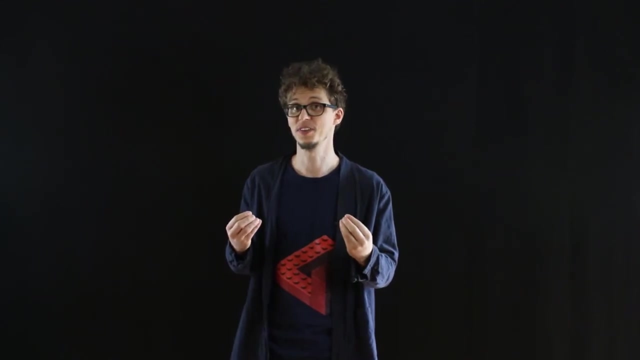 They can't see anything. They don't have any conscious level experience of having seen anything with their eyes, And yet they are able to accurately guess, with shocking accuracy, what they're looking at, Even though, if you ask them, Did you see anything? 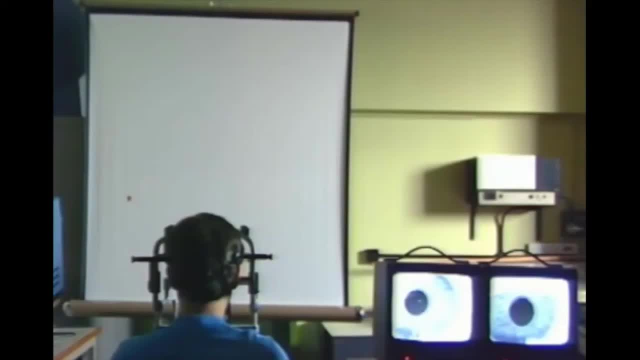 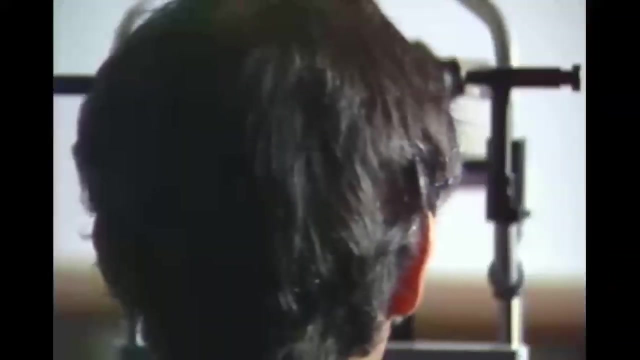 They will say: No, I didn't see anything, I'm blind. All right, Graham, can you tell me what sort of experience you had that made you move your arm? I just know something's moving over in the right field. Can you describe it? 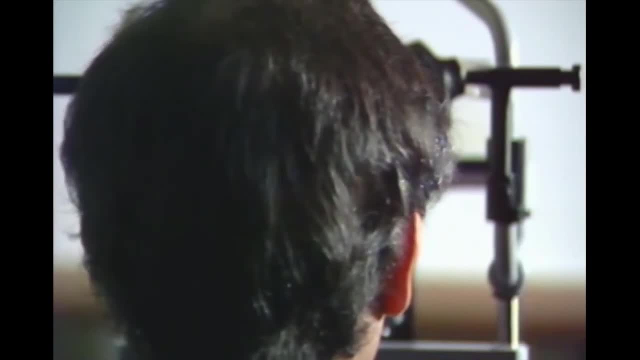 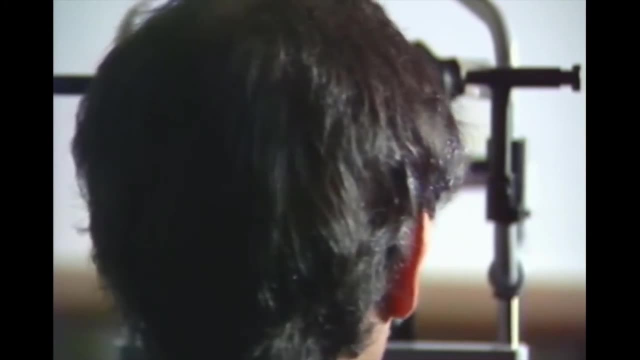 No, it's just. I know something's. there's some movement there. What did you actually see? I didn't see anything, Just an impression. It was just. I was aware that there was an object moving, yes, But could you describe the object? 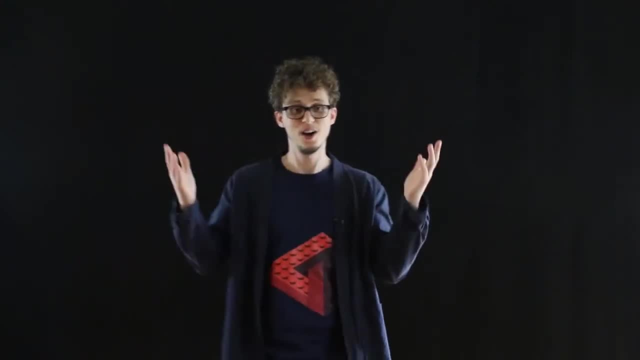 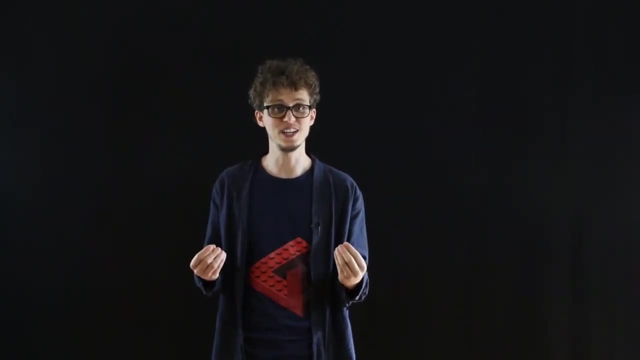 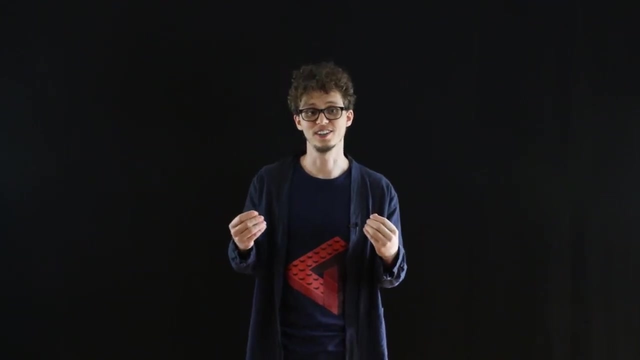 No, Okay, thank you. How does that work? How is that even possible? They're able to detect things with their eyes even though they don't have any experience of actually seeing anything, So their conscious vision is disrupted, whereas their unconscious vision is intact. 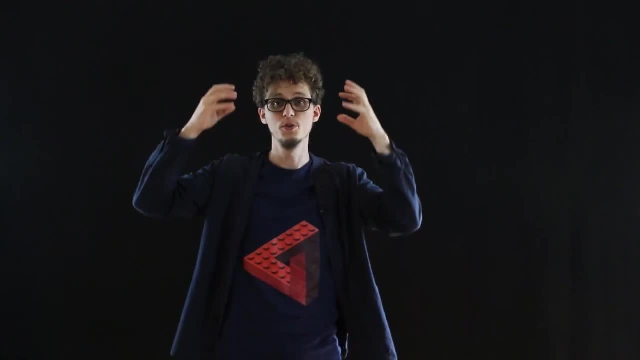 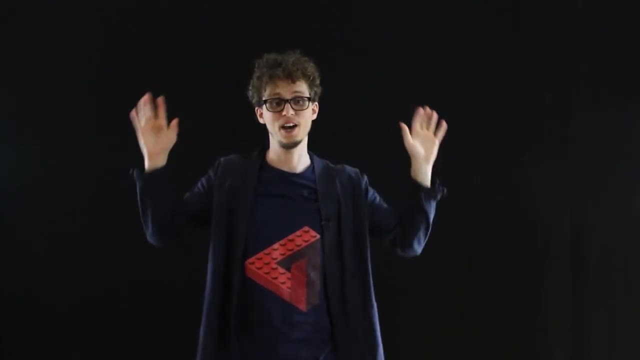 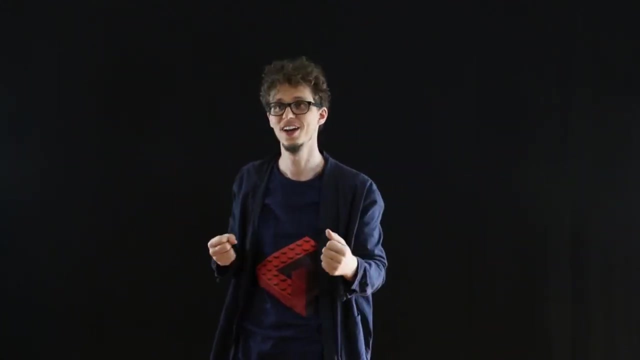 Visual input is going through their eyes, down the optic nerve, through the geniculostriate pathway, to the back of their brains, in V1. And that's where the pathway goes completely wrong. There's damage in V1 that causes them to not be aware of what they are experiencing. 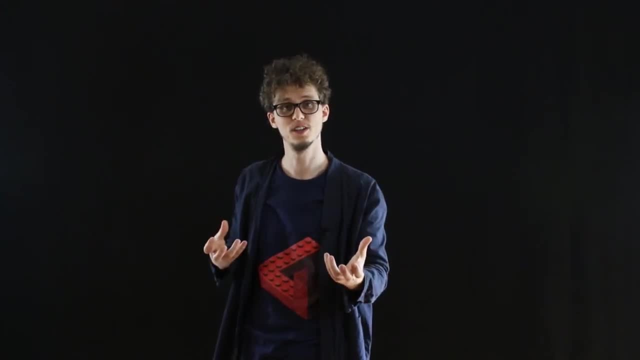 There is something wrong with their perception, So their sensation is intact. The information is getting into the brain through the eyes. It's being transduced, but it's not being perceived. Something has gone wrong with the perceptual process that builds this into an understanding. 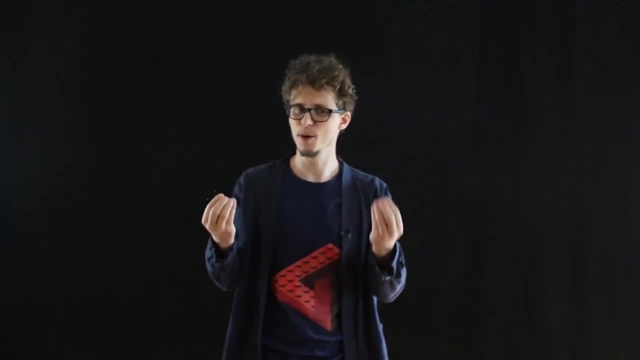 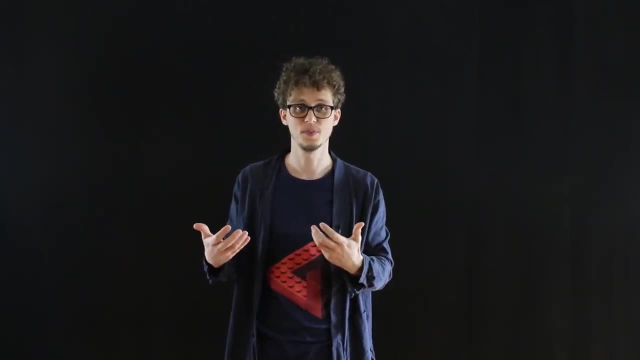 of the world. So fascinatingly, they still have some access to that information, but they don't have nearly as much access as a person who doesn't have blindsight, a person who has full use of their vision. We have a full, conscious experience of the world around us that we can describe in visual. 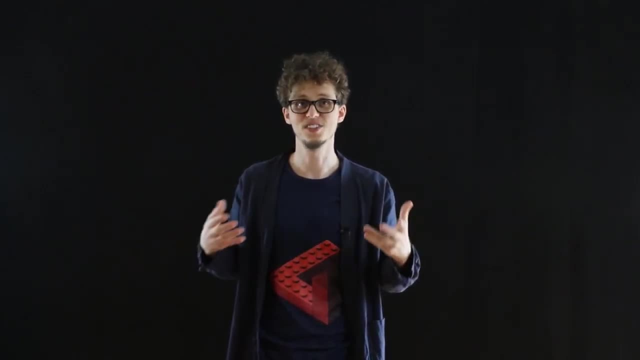 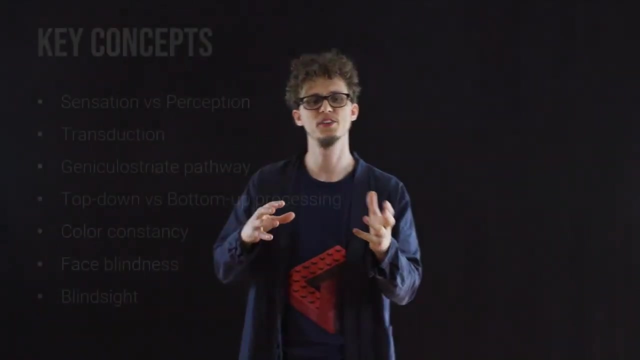 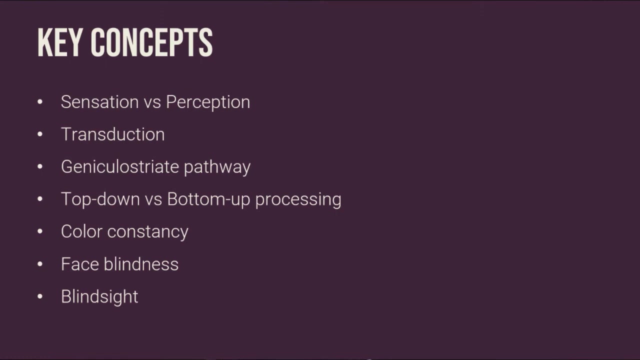 terms. A person with blindsight can't do that, But somehow they can still use some of that information to influence their behavior. Okay, so in this lecture we talked about the difference between sensation and perception, The idea that sensation is just the detection of stimuli, the detection of information from. 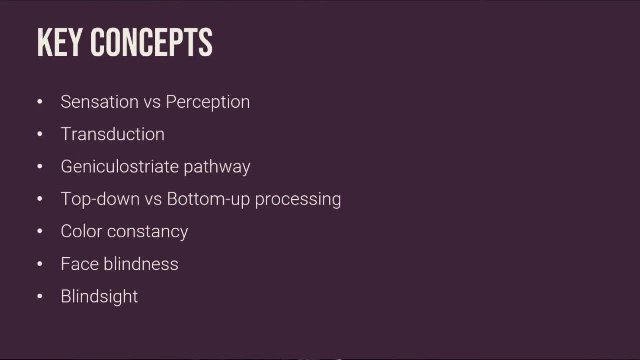 the outside world, whereas perception is more about understanding or interpreting that information. Transduction is the first step in this process, where we take information through our senses and we transform it into a format. It's a format that our brains can understand. Visual input, in particular, follows the geniculostriate pathway, going down the optic nerve back to 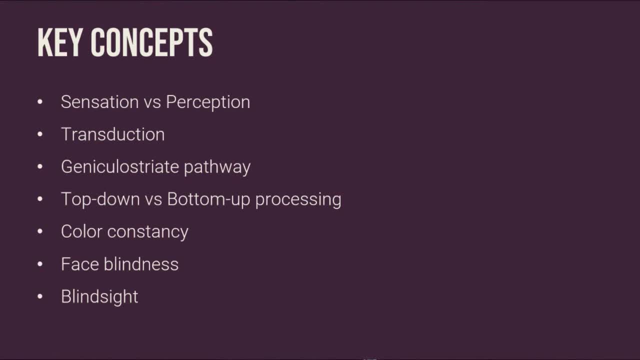 V1, in the back of the brain. We talked about top-down versus bottom-up processing. Top-down, using knowledge about the world allowing us to make predictions and fill in missing information. Bottom-up, in which we just take information from our senses and we use it to build a representation. 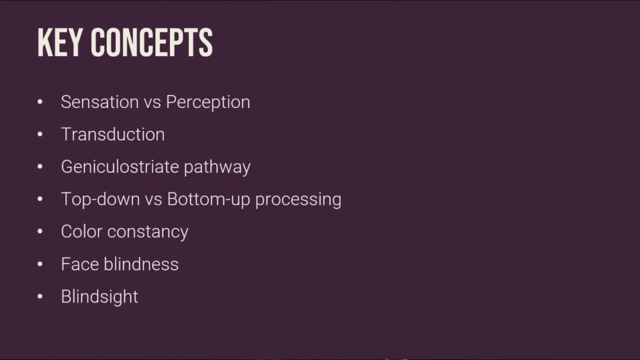 of what we are seeing And we talked about some of these perceptual processes, Some of those top-down effects Like color constancy illusions, And we talked about some conditions that elucidate the difference between sensation and perception. People with face blindness can sense faces. 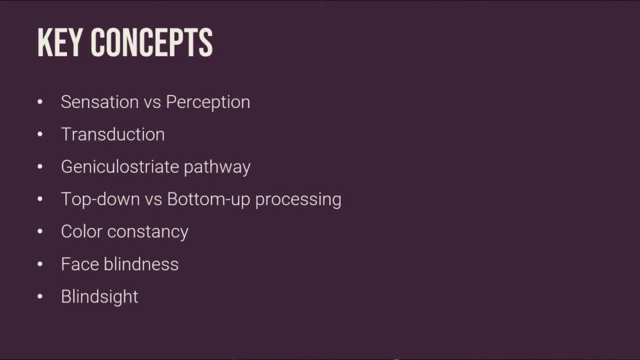 They can see all of the parts, But there is something wrong with the perceptual process of binding those parts together into a whole. There is something wrong with the way in which they understand or recognize faces. People with blindsight present an even more extreme version of this, where they have full 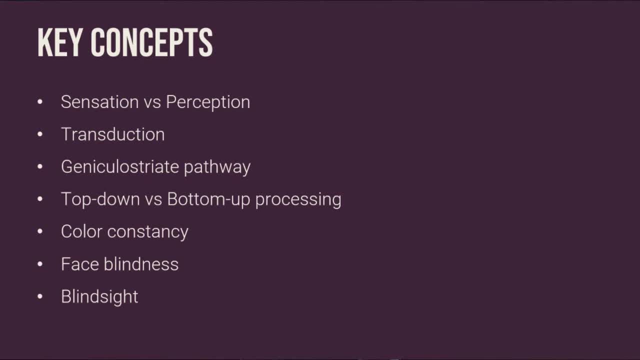 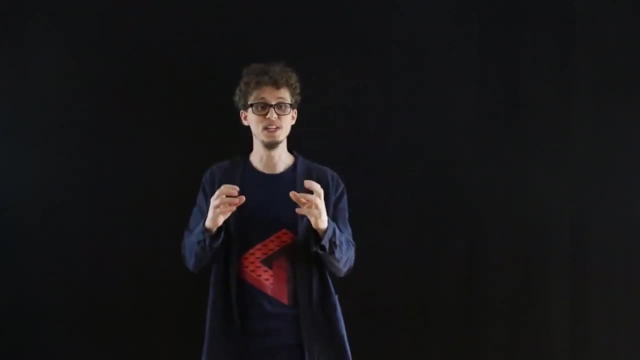 sensation through their eyes, But they don't have any conscious level perceptual experience, And yet somehow that information still gets into their brains and allows them to make decisions and act on the information that's coming in through their visual system. In the next lecture we'll talk more about mental imagery. 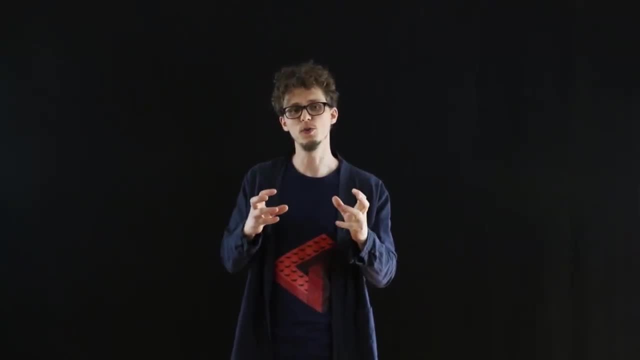 We'll talk about imagistic representations and what we can do with information once it's entered into our minds- Not just how we see things, but how we can manipulate the information in our mind's eye. Subtitles by the Amaraorg community.